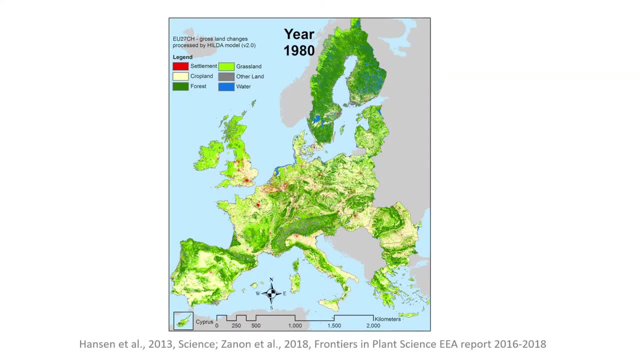 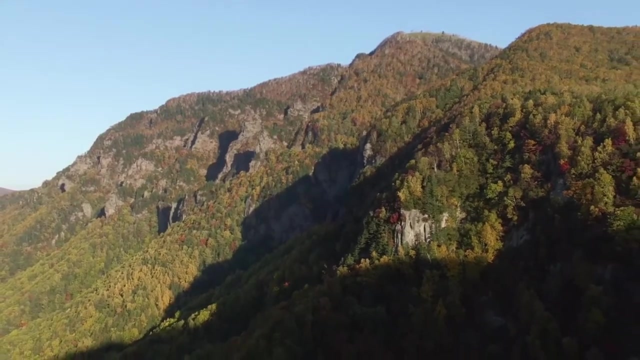 considered, And, as you might remember from previous lectures, nearly all forests in our region were cut at some point In the past, therefore disturbed. for millennia, natural processes such as tectonic uplift, volcanic climate erosion and sediment transport have shaped the earth's surface. However, 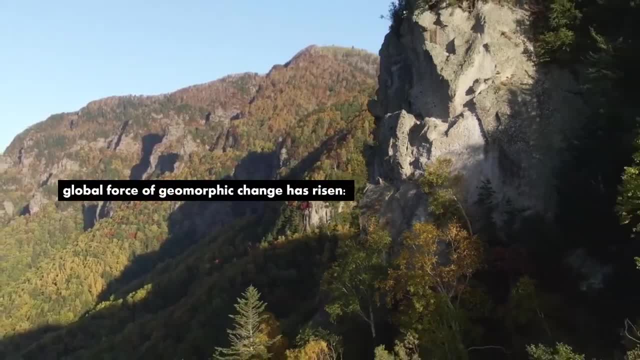 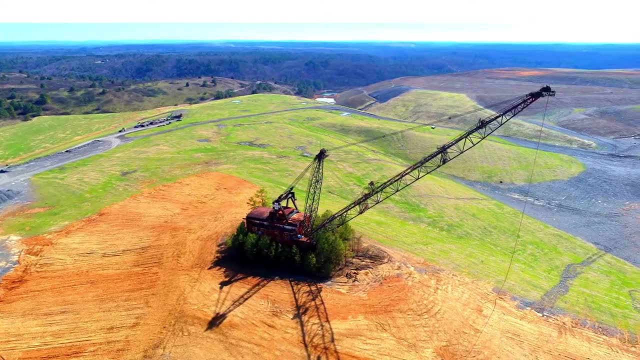 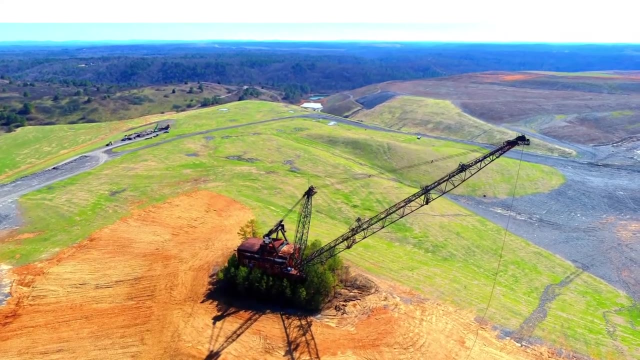 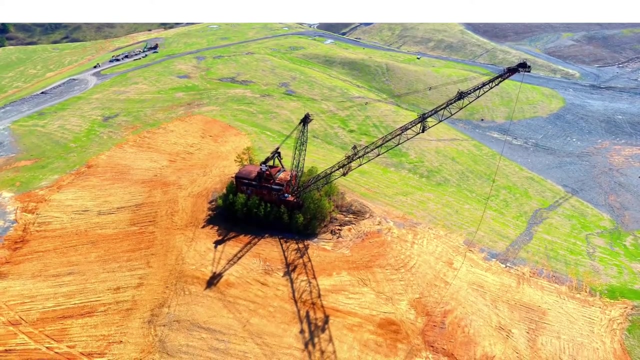 in the recent history, a different global force has been raised, and this is obviously humanity. Anthropogenic landscape now cover an extent of earth's land surface as many as many other globally important ecosystems. In these landscapes, human activities create characteristic geomorphic features, For example channels of irrigation, tourist systems on hill. 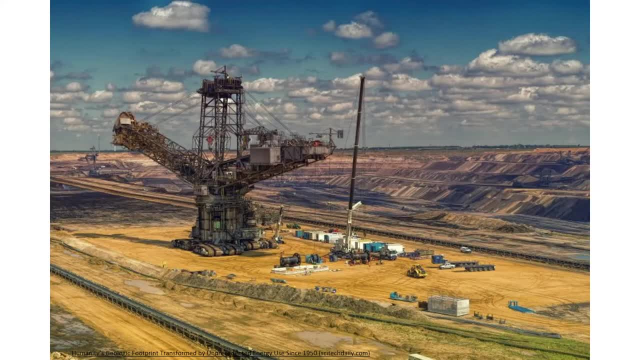 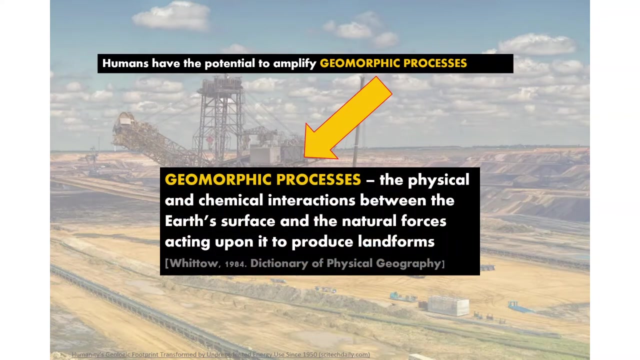 slopes, surface mining, And these features can significantly, significantly affect earth surface processes- Example: erosion, runoff, sediment transport and deposition. And humans have the to amplify geomorphic processes. Geomorphic processes as such, they are the physical and chemical interactions between the Earth's surface and the natural forces acting upon it. 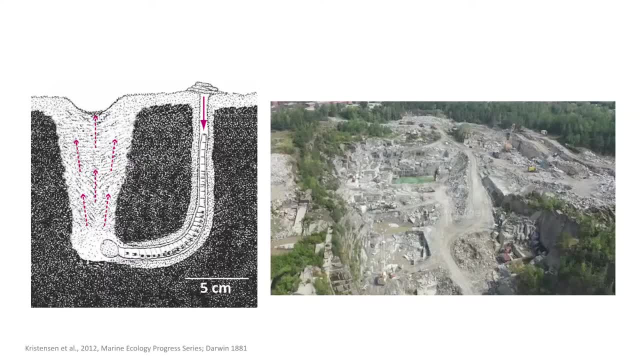 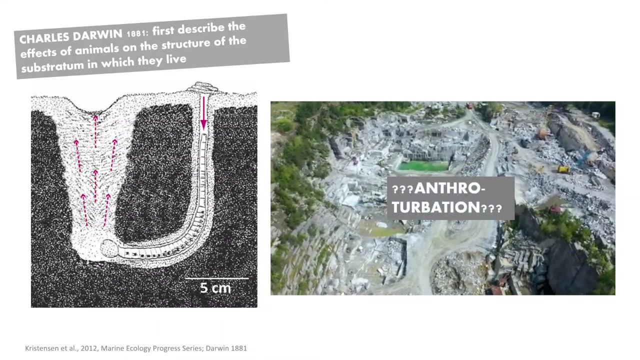 to produce landforms. It is maybe odd, but we can consider humans as bioturbant agents. Charles Darwin was the first to describe the effects of animals on the structure of the substratum in which they live. today, With this term, it defines as the reworking of soils and sediments by animals or plants. 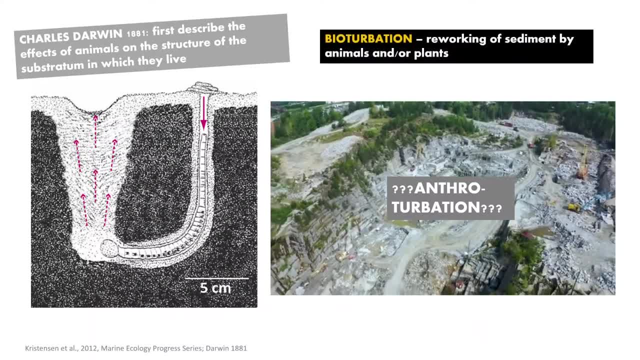 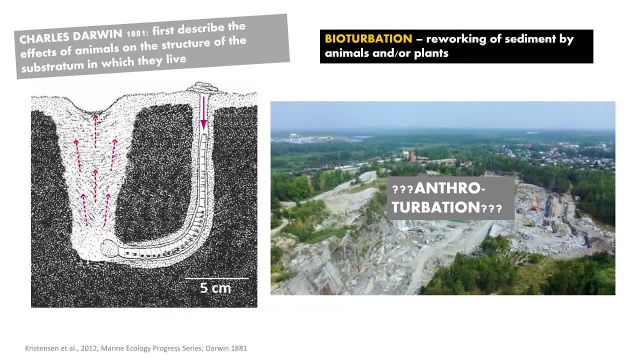 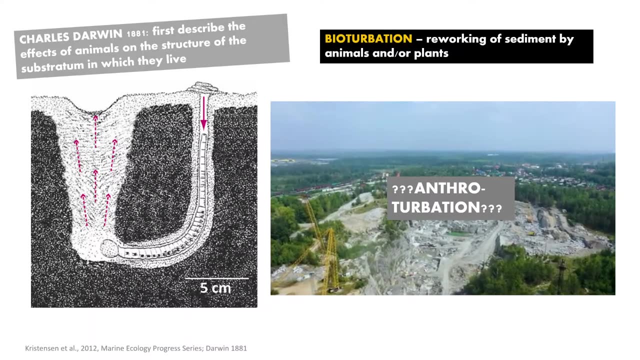 and bioturbation by humans, if we can call anthropoturbation, is a phenomenon without precedent in the Earth's history. Humans have become the dominant element in many Earth's surfaces, processes at different scales to the point that human activities can be considered distinct from but comparable to the effects. 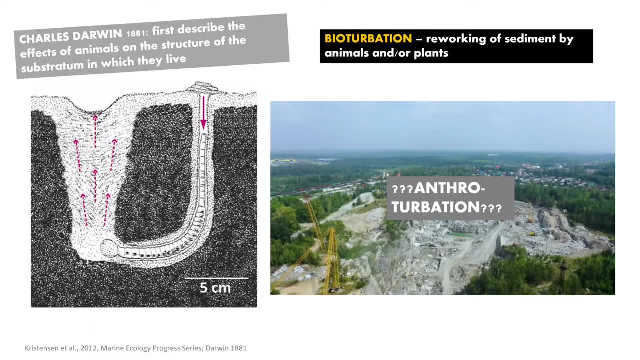 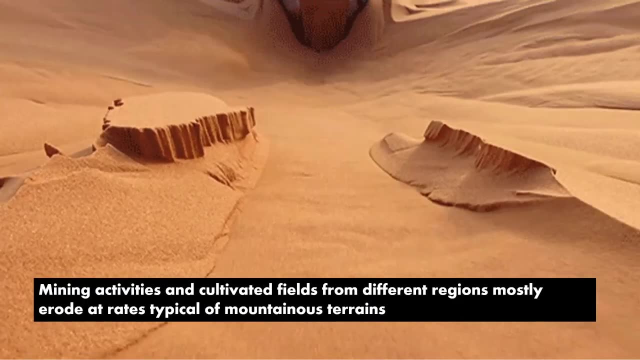 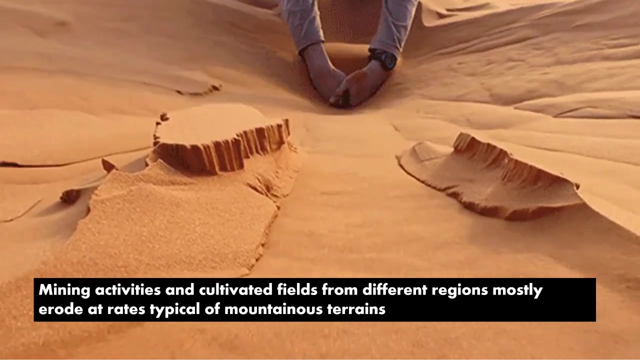 of climatic or tectonic transformations. Humans move increasingly large amounts of rock and sediment during various construction activities and therefore are a geological agent. Erosion rates from mining and agriculture that are among the highest rates in the general world are high. This in general, can exceed the rates of most natural erosion processes. 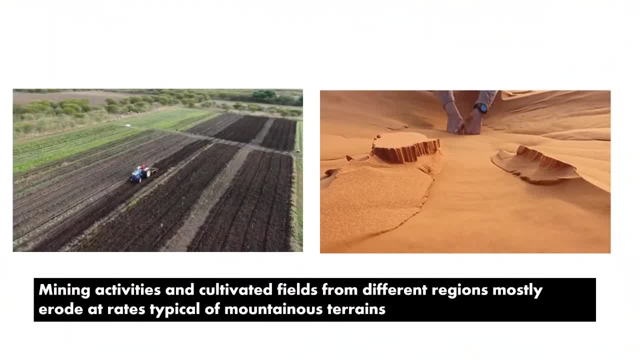 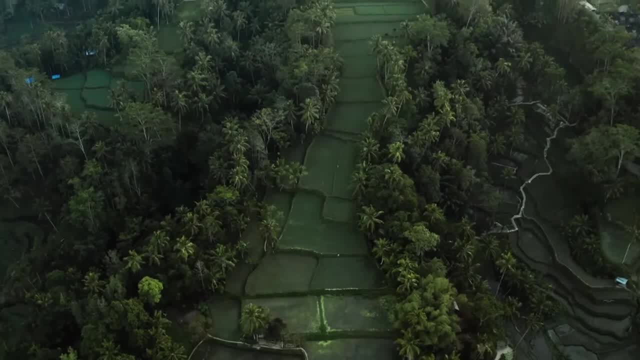 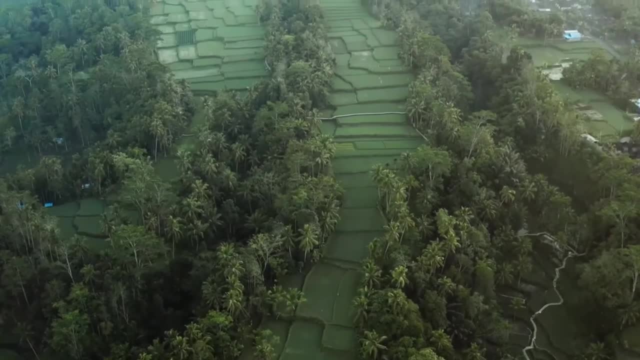 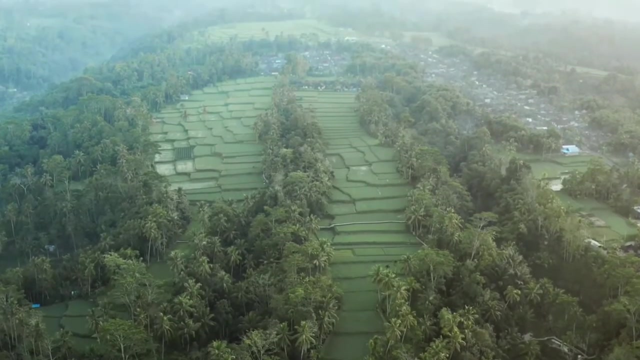 Mining activities and cultivated fields from different regions most likely erode at rates typical of mountainous terrains, for instance. so agricultural terraces are among the most evident and extensive signatures of humans on different landscapes of the world. Since ancient times one can find agricultural terraces. 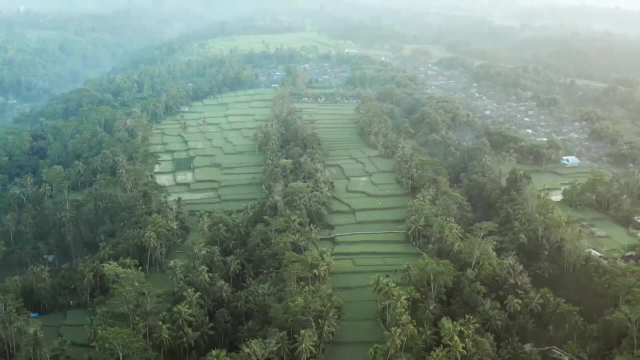 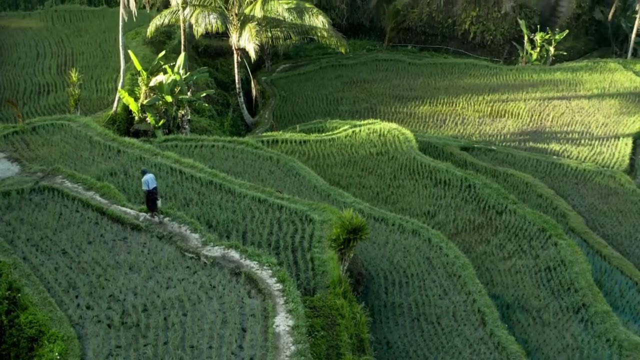 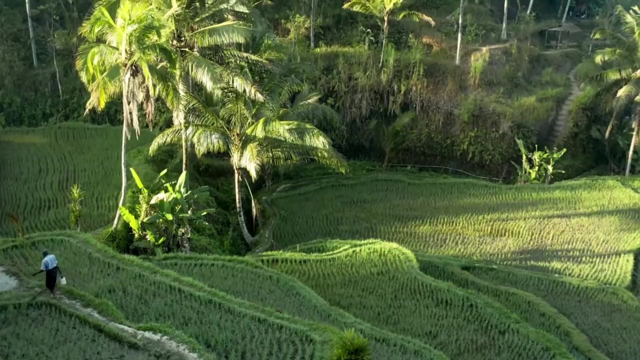 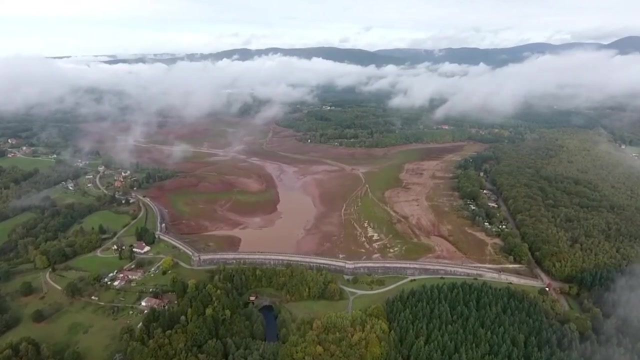 in different topographic conditions and used for various crops. Agricultural terracing introduced several critical issues: increase of slope failures and hydraulic erosion processes and redistribution of chemicals. Human impacts in floodplain modify the spatial distribution and the rates of hydraulic and geomorphic processes, and this might result in 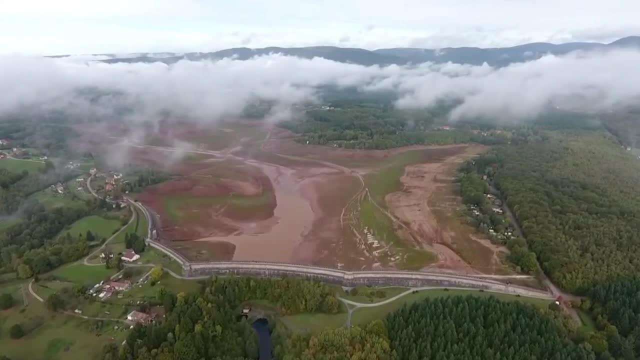 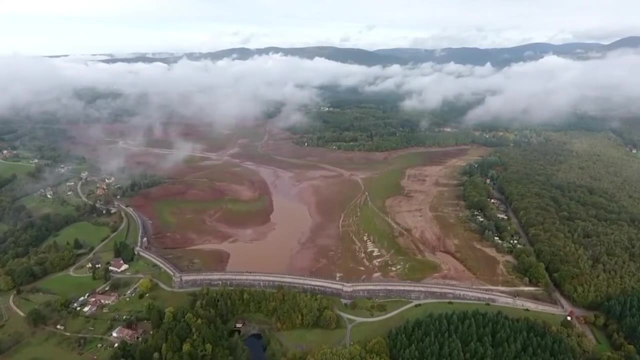 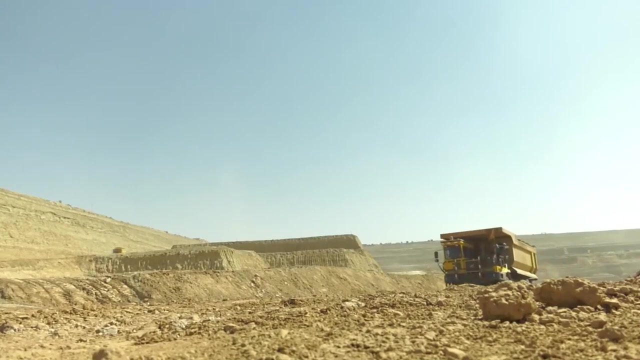 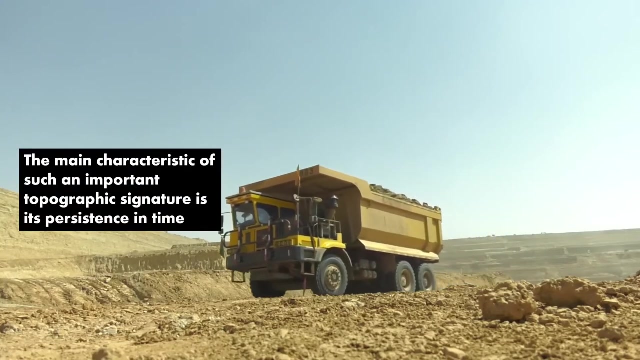 land degradation and deforestation. Geomorphic changes in geomorphology respond to several complex and interdependent factors. For instance, mines, quarries, urban areas and all types of infrastructure represent an estimated 13% of such changes. Compared to other anthropogenic topographies, mining occupies a relatively smaller amount of 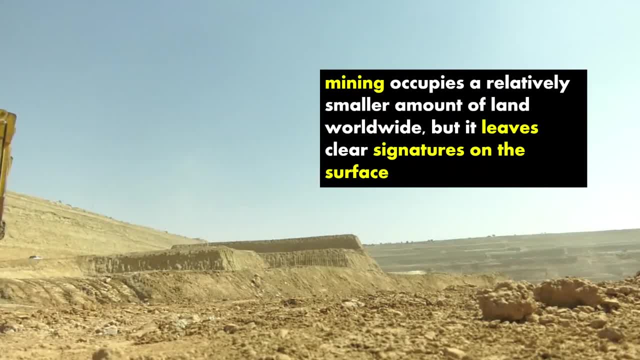 land worldwide, but it leaves clear Signatures on the surface. The main characteristic of such an important topographic signature is its persistence in time, so they can persist over the long time periods, With the extending of mining to large scales due to the mineral demands mining-related. 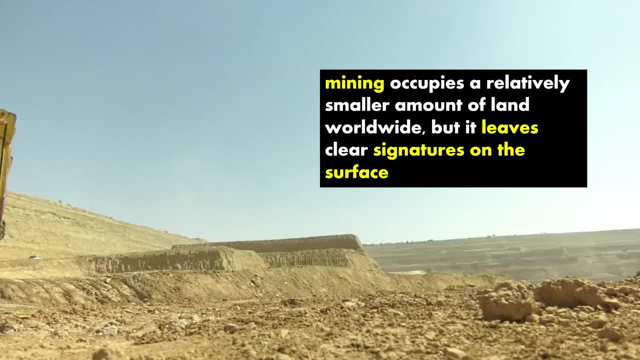 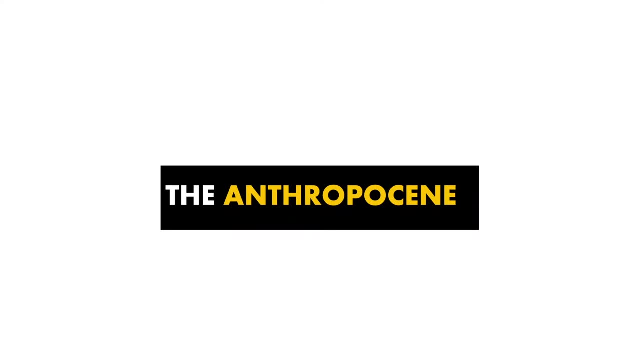 hazards and disasters in the earth's surface will become more and more severe, inducing risk Also for the landscapes surrounding the mines. Scientific community is now debating the fact that we are living in the new geological epoch, stratigraphically distinct from the Holocene, and that's why we call this the Anthropocene. 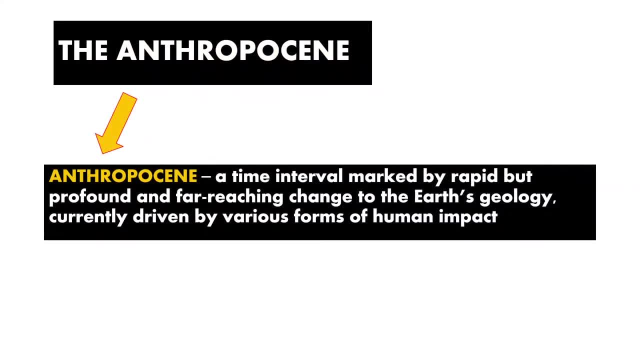 In common usage. the Anthropocene refers to a time interval marked by rapid but profound and far-reaching change to the earth's geology, Currently driven by various geological changes. the Anthropocene refers to a time interval marked by rapid but profound and far-reaching change to the earth's geology, Currently driven. 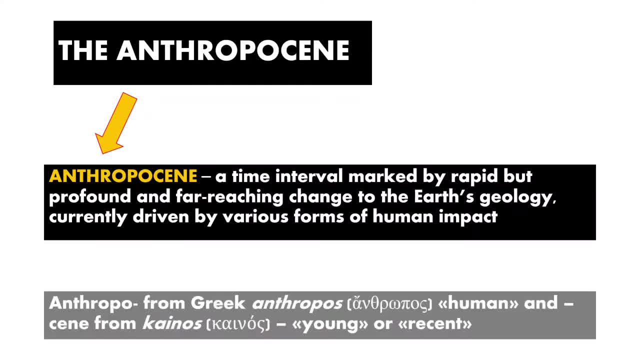 by various geological changes. the Anthropocene refers to a time interval marked by rapid but profound and far-reaching change to the earth's geology- This term is manifestly Furyal之後 by various forms of human impact. But where did the Anthropocene come from? 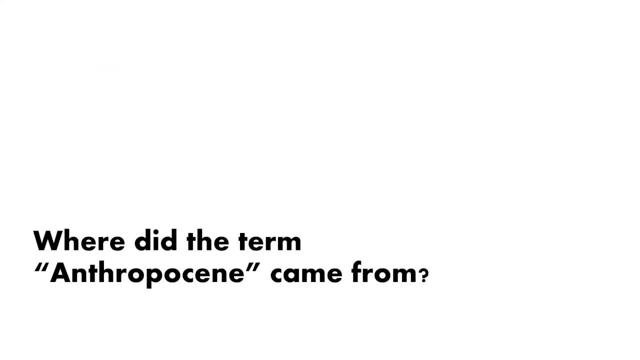 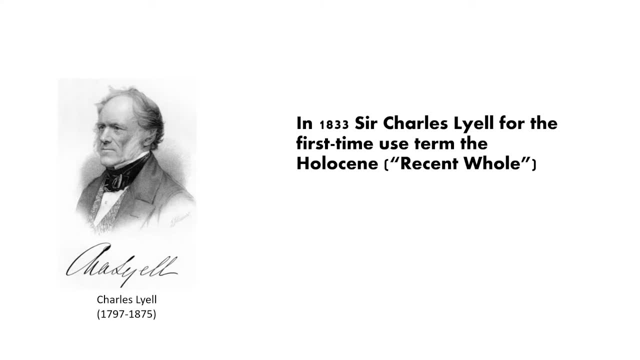 To get to the term Anthropocene, we first need to return 200 years to the past. It was Charles Lyell who for the first time used term Deholocene- Recent whole, therefore. he put a certain foundation of how we name the time in which we are living. 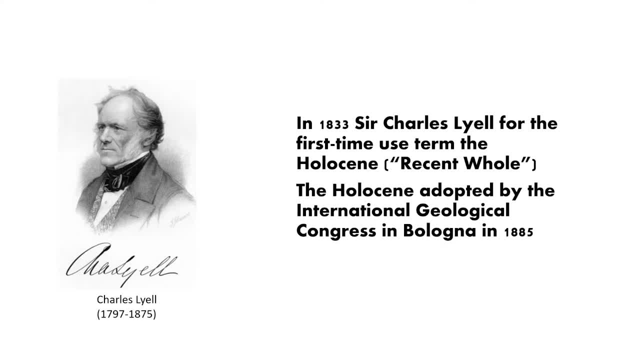 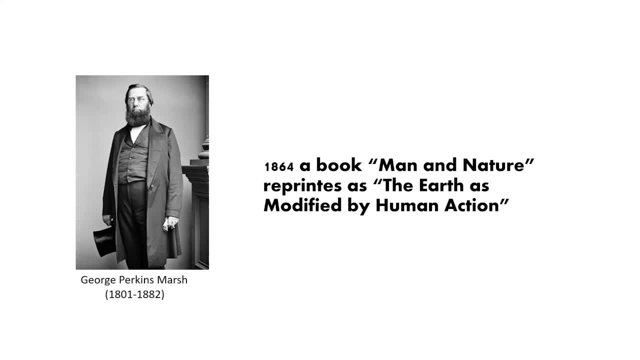 now, Yes, Age, future and outcome: material creation and discovered population of living creatures, Go mode and geographic evidence indicated that during the Holocene, mankind's activities gradually grew into a significant force, as recognized early on by a number of scientists, For instance, 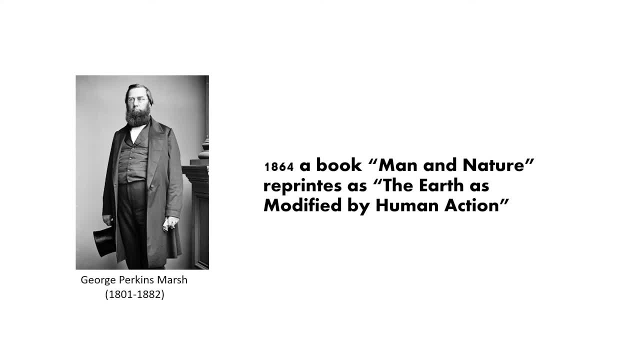 George Perkins Marsh, on 30 September 1847, gave a lecture to the Agricultural Society in Vermont, USA, where he talked about the human impact. His ideas later were published in a book titled Man and Nature. More than 160 years on, it really does pay to reread his work, as it seems remarkably. 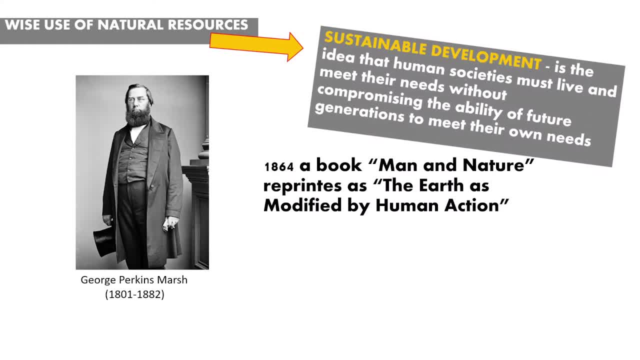 actual today. It also shows that he was decades ahead of most of other thinkers on this subject. After all, he delivered his lecture a decade before John Tyndall began to explore the thesis that slight changes in the atmosphere's composition could cause climatic variations, And it was a full half a century. 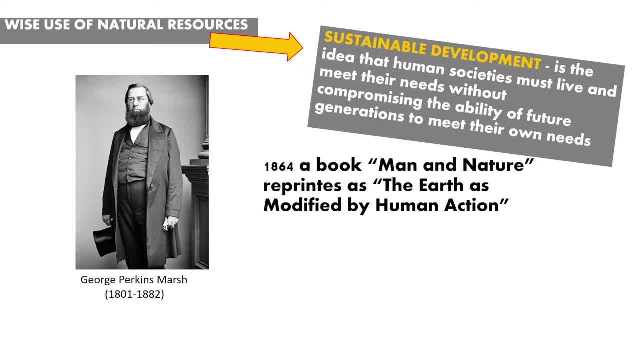 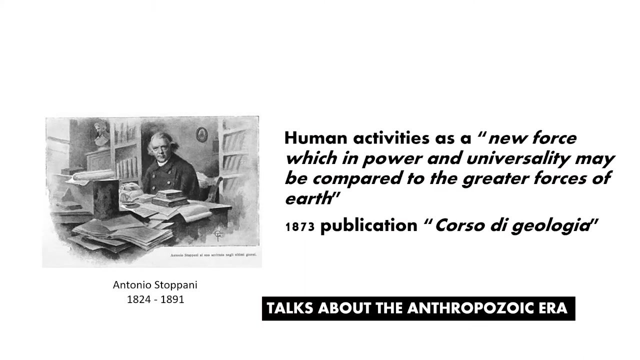 before Suente Arrhenius proposed that carbon dioxide emitted by the enormous combustion of coal by our industrial establishments might warm the world. Marsh was not an environmental scientist, but he believed that all consumption must be reasoned and considered, with the impact on future generations always kept in mind. Antonio Stoppani, a founder of Italian geology. 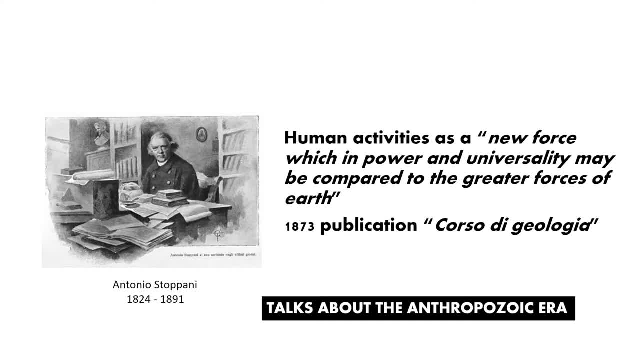 and also paleontology, I would say also in geo-archaeology, rated mankind's activities as a new force which, in power and universality, may be compared to the greater forces of the earth. Stoppani already spoke of the Anthropocene era and thus determined Anthropocene as 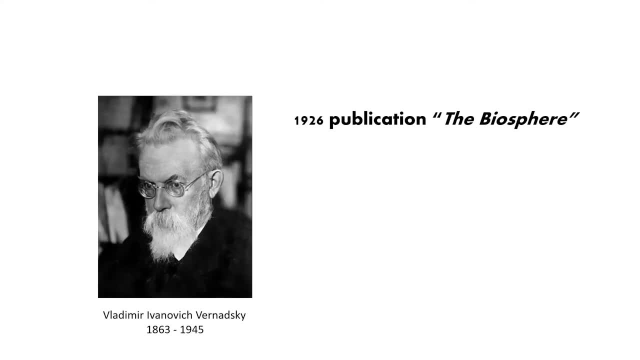 such, Vernadsky, the founder of Geochemistry and BioChemistry, in 1926 recognised the increasing power of mankind as the part of the biosphere and he wrote: The direction in which the processes of evolution must proceed, namely towards increase or development, should be heavier, but not less than or equal to, in concert with**** and 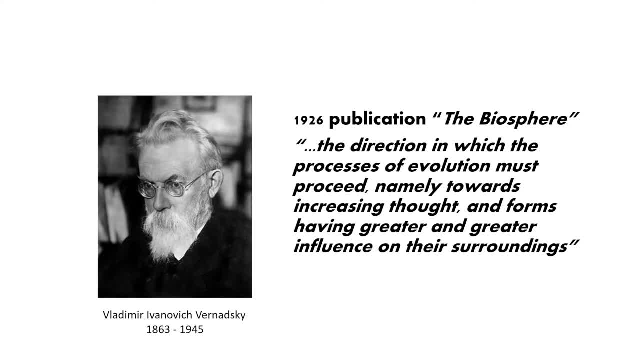 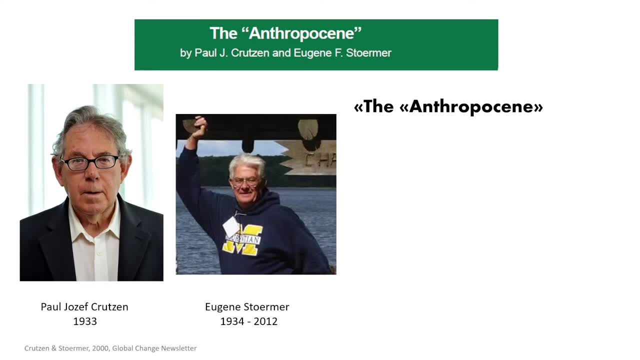 energy. we must still counteract sao-nite's agony and שא�i day-and-day wounds. but he" thought and forms have greater and greater influence on their surroundings, so he were underlying the force of human. In 2000, Paul Crutzen and Eugen Steuermann. 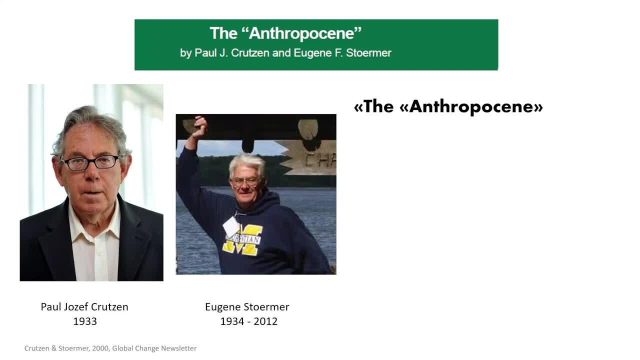 proposed that human modification of the global environment had become significant enough to warrant termination of the Kern-Hausen geological epoch and formal recognition of the new Anthropocene epoch. Unfortunately, Paul Crutzen died in 2021, therefore both these authors are gone, but their 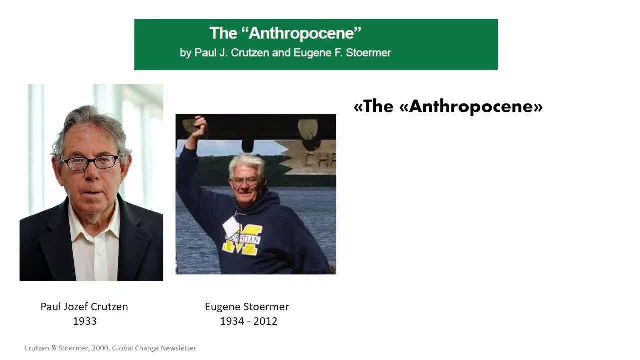 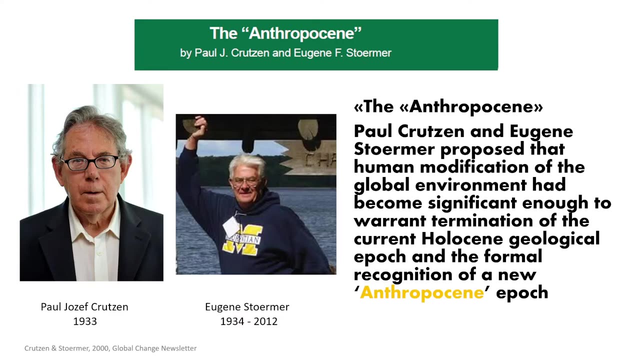 legacy is still ongoing, especially when we're talking about the Anthropocene, Although their term Anthropocene was not new. they cite a number of similar proposals for terminological recognition of human dominance of the Earth's ecosystems that had been made of Earth's ecosystems that had been made of Earth's ecosystems that had been made of. 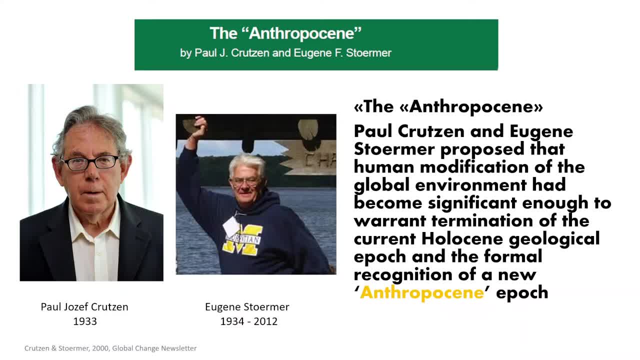 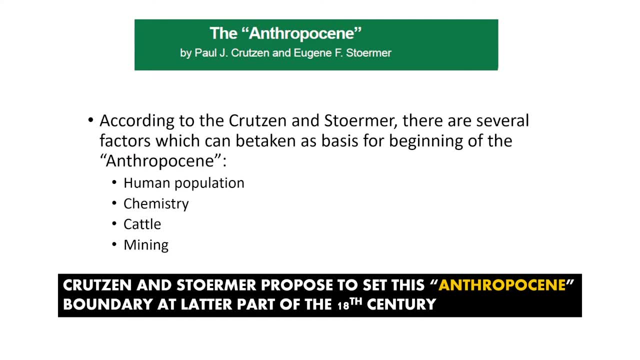 over the last 140 years or so. Crutzen and Steuermann proposed that there are certain points according to which the beginning of the Anthropocene can be set. These include human population, chemistry, cattle and mining. So let's unfold each. 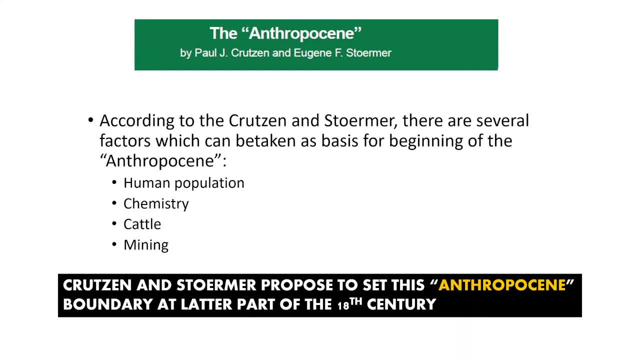 of these points more closely and begin with human population. Crutzen points correctly that the expansion of the Earth's ecosystems has been a significant step in the development of the. the expansion of the Earth's ecosystems has been a significant step in the development of the. 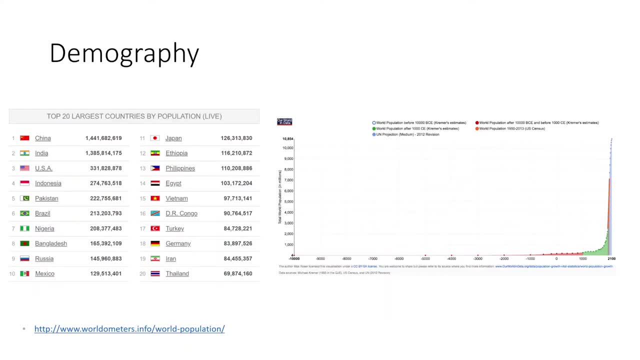 mankind, both in number and per capita. exploitation of Earth's resources has been astounding. To give a few examples: during the past three centuries, human population increased tenfold, ten times more than it was before, and these numbers are still increasing, as you are aware. This 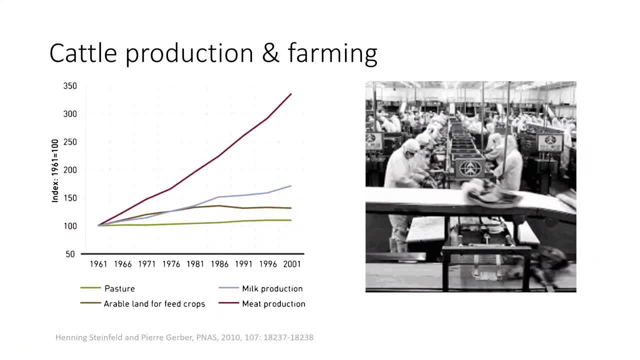 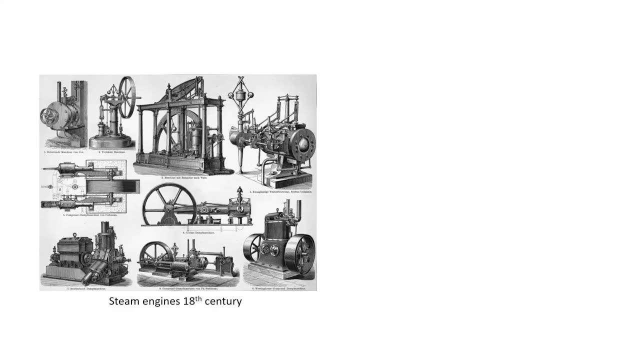 population increase is accompanied by growth in cattle breeding. It has been estimated that we utilize about one to two cows per average size family each year. Not to mention meat consumption is a rocket high at the moment. Crutzen and Steuermann underlined that over the last two 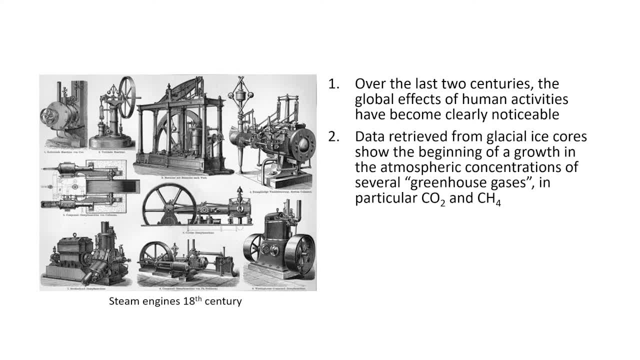 centuries, the global effects of human activities have become clearly noticeable. Secondly, data retrieved from glacial ice cores show the beginning of growth in the atmospheric concentrations of greenhouse gases, in particular carbon dioxide and methane, and these changes coincided with James Watt's invention of the steam engine around well precisely in 1784.. As four points, 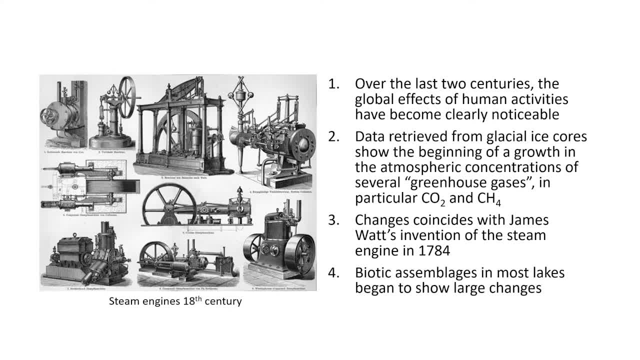 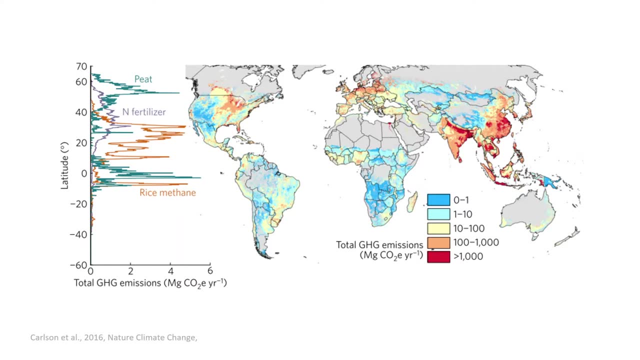 they mention, biotic assemblages in most lakes began to show large changes, so that means changes in lakes and aquatic ecosystems in general. Indeed, several climatically important greenhouse gases have substantially increased in the atmosphere, such as carbon dioxide by more than 30% and methane by even more than 100%. 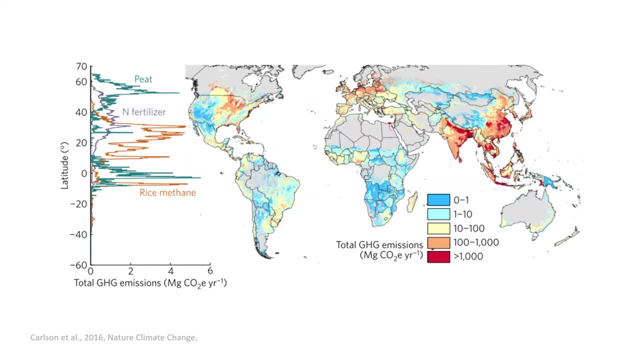 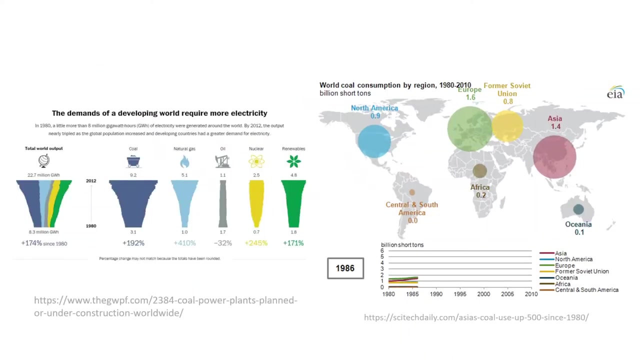 More. nitrogen is now fixed synthetically and applied as fertilizers in agriculture, then fixed naturally in all terrestrial ecosystems. so that shows the shift from the natural to human related neutral fertilization. Furthermore, the release of CO2- globally- about 160 tg per year- to the atmosphere by coal and oil burning is at least two times larger than 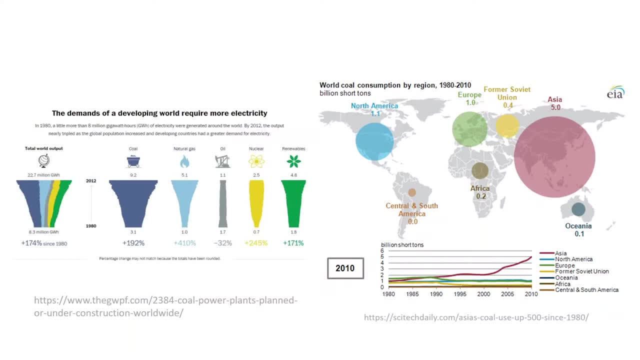 the sum of all natural emissions occurring mainly as marine sulfides from the oceans, Not to mention volcanic eruptions. as we can see in the video above, This is due to the fact that carbon dioxide is already present in water, so now it could be said that carbon dioxide is the JO 17.. 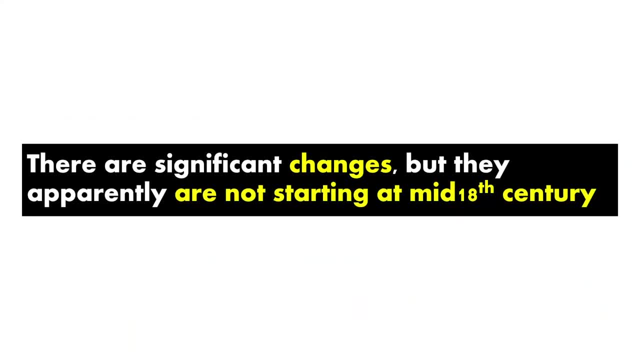 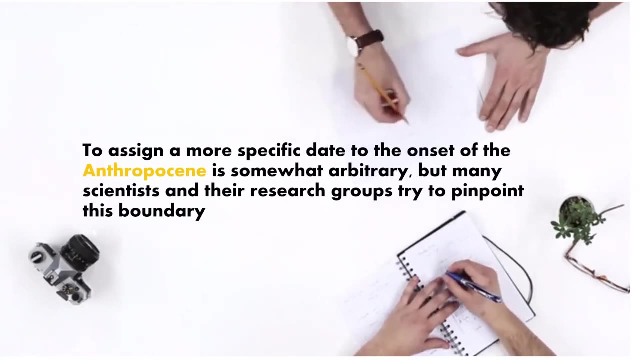 There are significant changes, but they cannot be set starting at the mid-18th century, as these authors claim. To assign a more specific date to the onset of the Anthropocene is somewhat arbitrary, but many scientists and their research groups try to pinpoint this boundary. 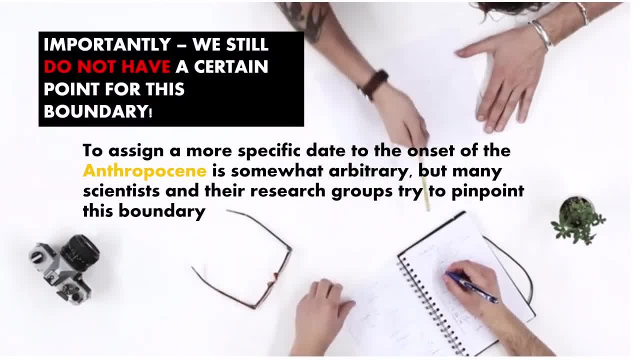 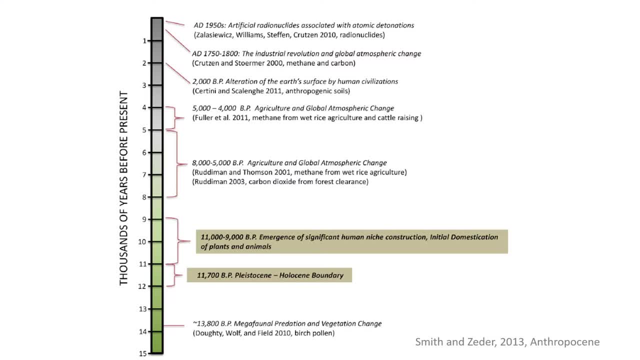 Importantly, we still do not have point for this boundary. Alternative temporal boundaries for the Holocene and Anthropocene boundary do exist, but each of them have both pros and cons, meaning they all have some link to human activities, but only few of them. 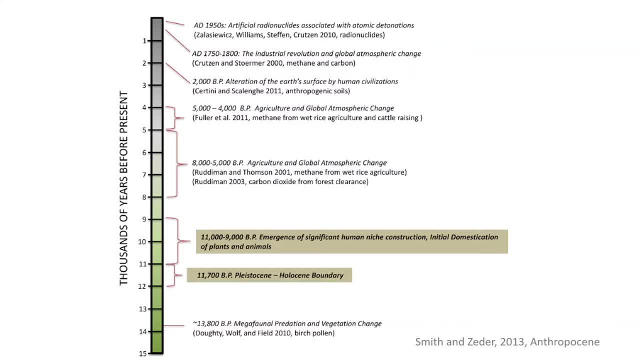 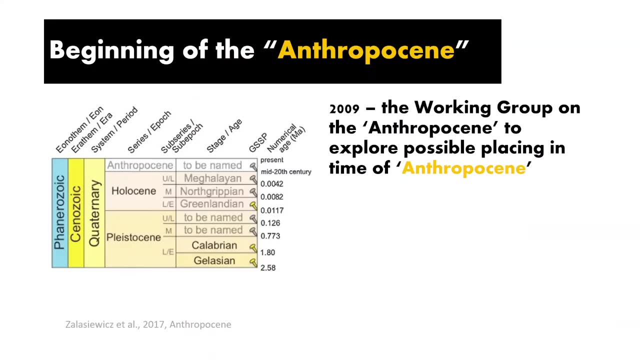 actually could be real candidates. In 2009,, the Anthropocene Working Group of the Sub-Commission of Quaternary Stratigraphy was established to consider the evidence for environmental signatures that could be uniquely attributed to a new epoch, and this working group is responsible for. 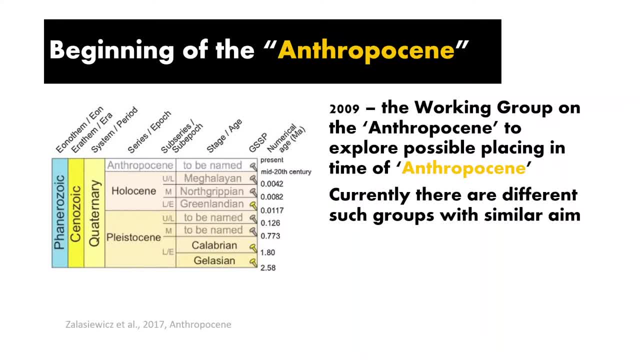 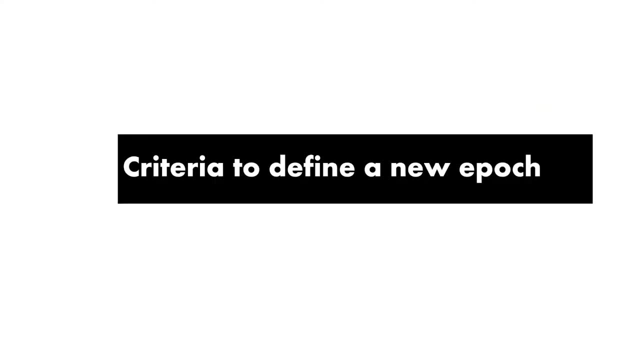 producing a recommendation to be considered by the International Commission on the Stratigraphy, including a requirement for defining its lower boundary. You see, there is a certain way how new boundaries are defined and there is a certain way how new epoch as well, as we call it in geology, can be defined. It is not enough if one. 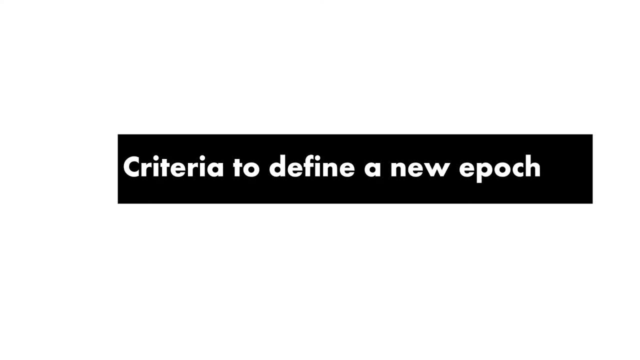 scientist published an article on this topic and says that he thinks that the Anthropocene started in mid 18th century or other time period. There are certain protocols to fulfill at first and to meet a consensus within the worldwide scientific community, after which such new epoch actually can be established. 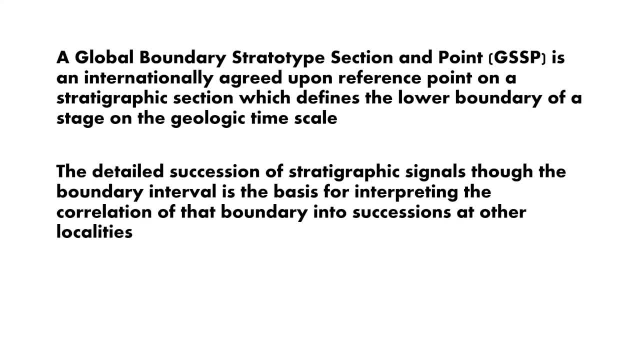 The recognition of human-induced stratigraphic marker that may underpin certain stratotype or point or so-called golden spike with which to define the lower boundary of the new epoch, is essential to this process and hence the definition of the Anthropocene itself. A global boundary stratotype, section a. 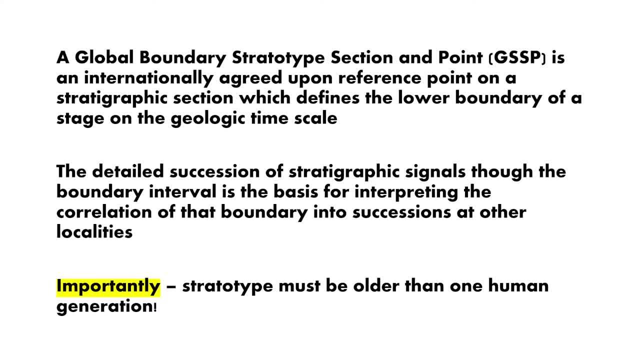 point, or abbreviation GSSP, is an internationally agreed upon reference point on a stratigraphic section which defines the lower boundary of a stage on the geologic type scale, and majority of these points and sections are based on geochemical and paleontological changes And the detailed succession of 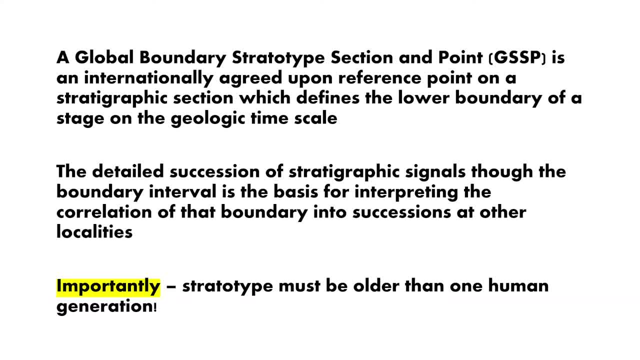 stratigraphic signals, although the boundary interval is a basis for interpreting the correlation of that boundary into successions at other localities. and, importantly, the stratotype must be older than one human generation. so that means there should be this fingerprint of changes traceable after several decades and lifespans of 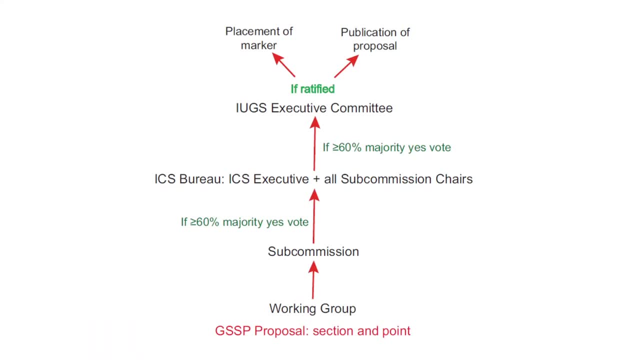 the humans. The whole process can be visualized in a rather simple scheme where it all begins with a GSSP proposal, then work within the working groups and sub-commissions. If at least 60% or more vote yes, the proposal goes further until it is ratified. 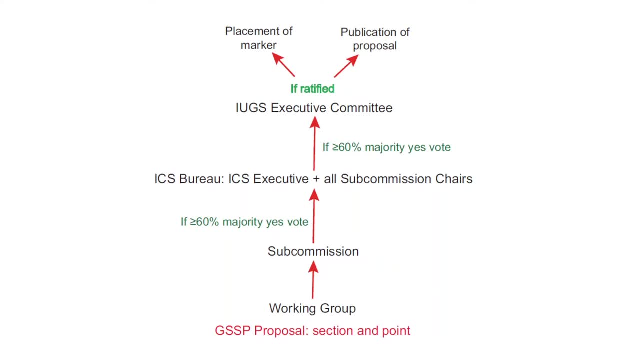 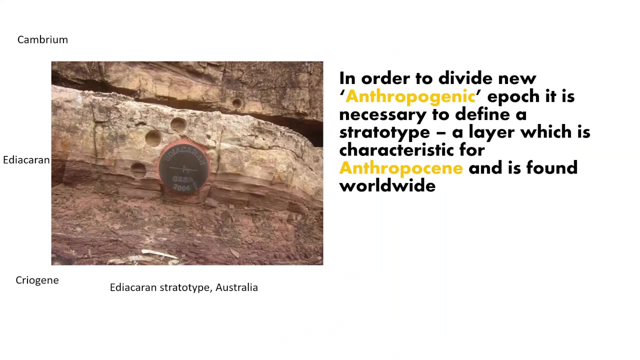 meaning changes are officially approved and used worldwide. In order to establish a new anthropogenic epoch, it is necessary to define a stratotype, a layer which is characteristic for the Anthropocene and is found worldwide. Unfortunately, lack of such precise layer forms a stage for various discussions. 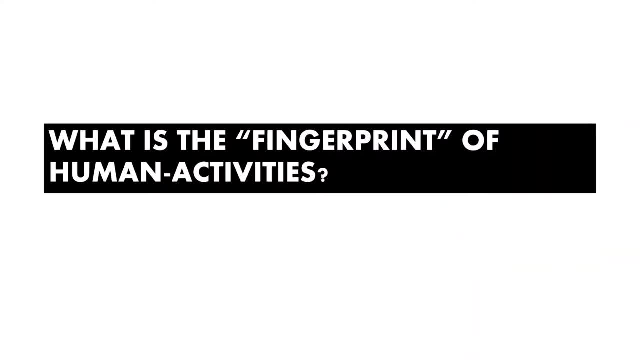 OK, so, as you know, the Anthropocene must be defined based on certain physical or chemical sediment characteristics, Based on what chemical element or object remains within the could establish the Anthropocene. Well, that's the good question, and let's look on some of these. 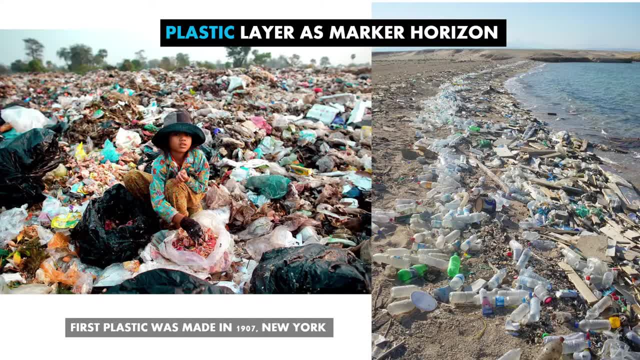 For instance, the rise of plastic since the mid 20th century, both as material element of modern life and as growing environmental pollutant, has been widely described. Discarded in various ways after use, we see plastic widely around us- as litter, unfortunately- And plastics might be. 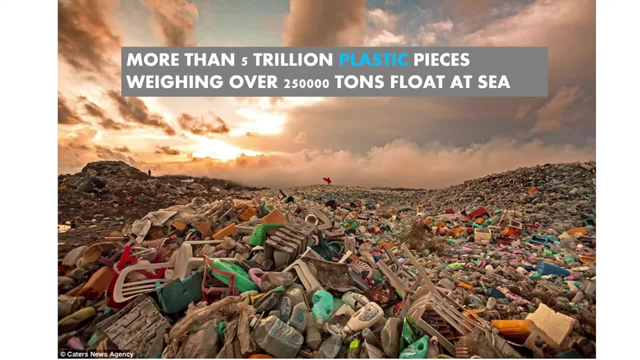 used as markers of the age and character of the sedimentary deposits that they are buried, Much in the way that geologists use, let's say, fossils to characterize the certain sediments. Therefore, plastics are relatively easily recognizable when they are used as a material element of modern life and as growing environmental pollutant. 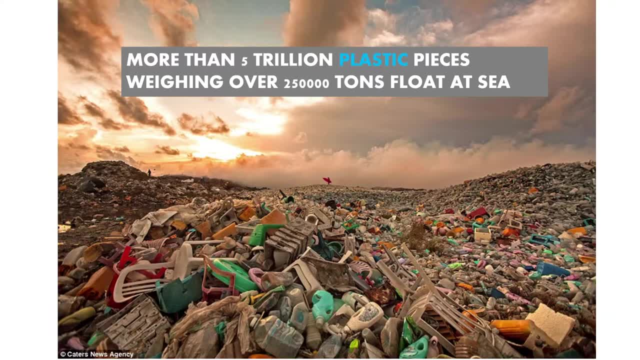 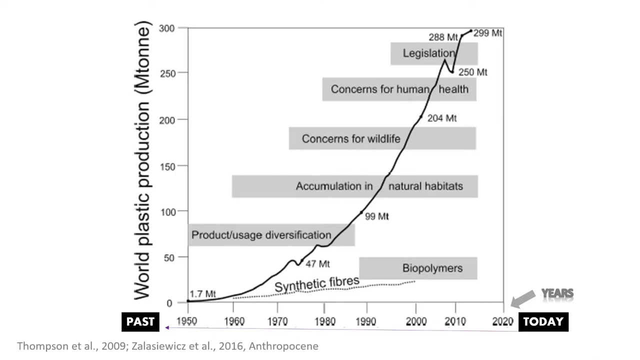 Large pieces without well we then we can recognize them without any sophisticated analytical equipment, but the plastic has this tendency to break apart in smaller and smaller pieces, and then we need really costly and sophisticated equipment to recognize these particles in the sediment. There has been a dramatic rise of produced plastics from the less than 2 million tons. 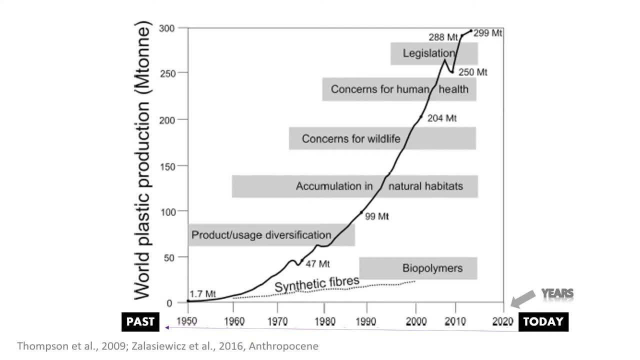 manufactured in 1950s to the 300 million tons made annually today. So these are enormous amounts of plastic what we are producing worldwide. Plus, I mean, the plastics are proving to be much more mobile than other human-made materials such as, for instance, glass or ceramics. 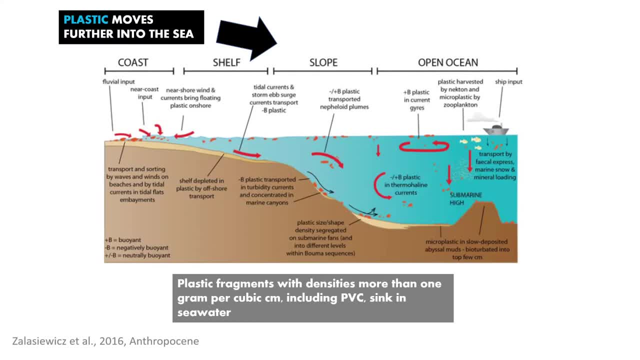 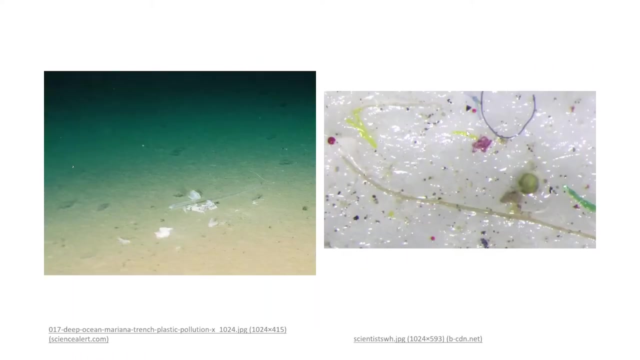 And uh um, plastic fragments with a density is more than one gram per cubic centimeter, including pvc sink, in seawater. They can then be moved in shallow water and by various gravity driven currents in deep water, before finally being deposited. It is hard to grasp, but the plastic can be found. 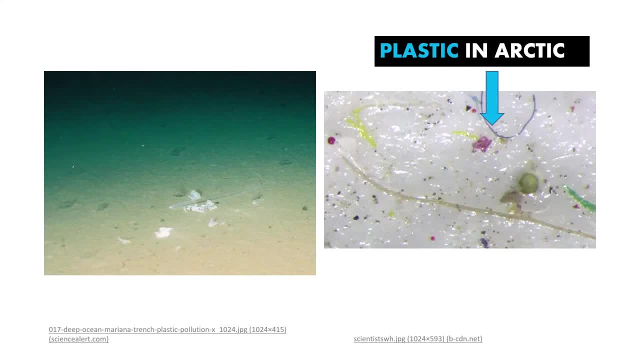 deep into the waters in arctic and mariana trench, which, as you know, nearly 12 kilometers deep depression in the ocean. so therefore we can say, yeah, we did it. we polluted with a plastic everywhere. so that's got a sad thing to think that our impact is so heavy on the nature. 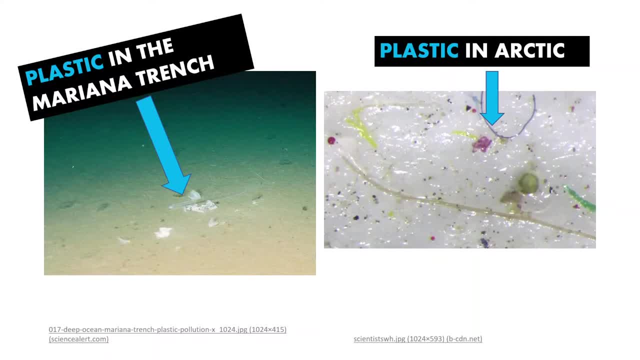 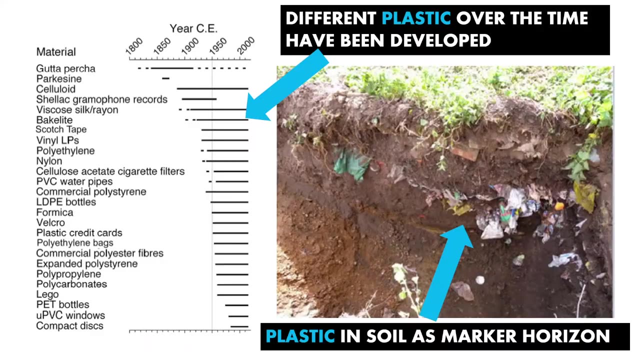 Plastic in arctic, plastic in deep oceans, in the snow in siberia, also in the air. plastic is transported by the air as well, and the geological longevity or the lifespan of the plastic polymers is poorly known, mainly because these are novel materials that have been in the environment. 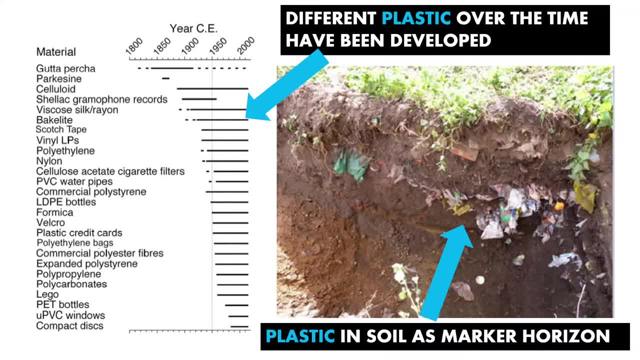 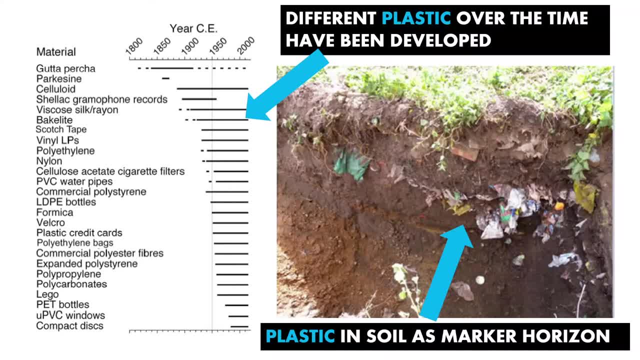 as as a marker, especially when the plastic is buried in the earth and the sunlight is not directly reaching the plastic, then the plastic can survive, let's say being kept and encapsulated into the, in the, in the sediment, while if it's open air storage, then the plastic comes. 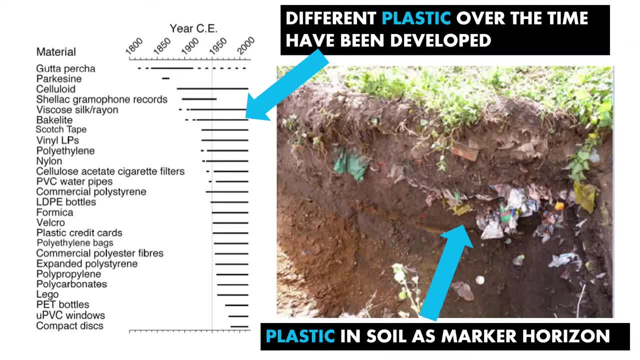 back into the air and then it's broken into smaller pieces, as i mentioned. However, there are also other scientific discoveries that there are indications that certain microbes degrade plastic. but this is this. scientific research is still in its early stages, so it's too early to say that nature itself will consume the plastic. 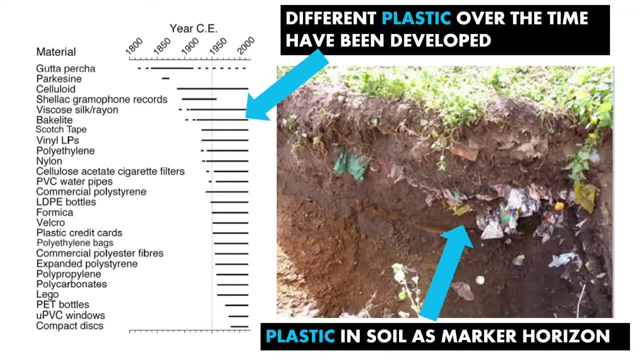 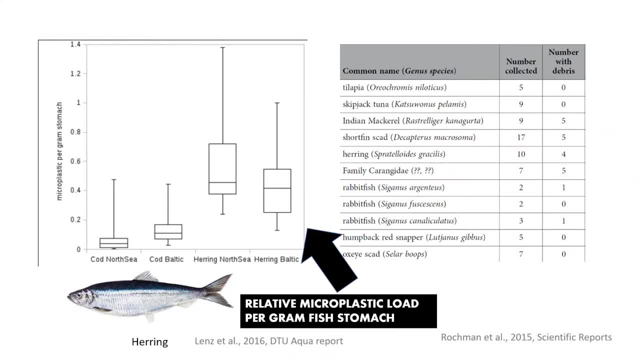 So we still need to care out carefully what we are doing with the plastic. It's worrying because anthropogenic debris, including plastic, found in wildlife, raise some concerns. Vast amount of seafood rich in plastic debris is on the sale for human consumption and there are scientific 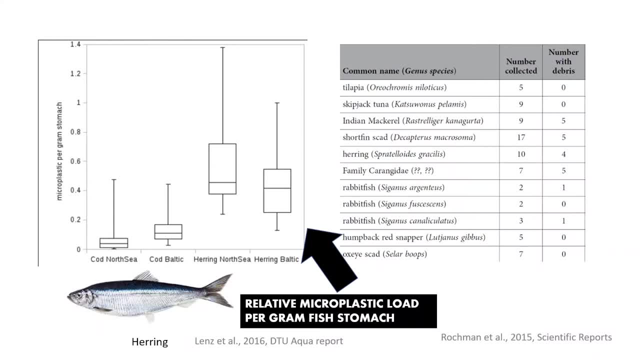 publications also on that. we can find microplastic also in placenta of, of, of uh, nearly born child mothers, and therefore the plastic can transform into the human body as well. Well, if we talk about the debris, then in in Indonesia anthropogenic debris has been found in: 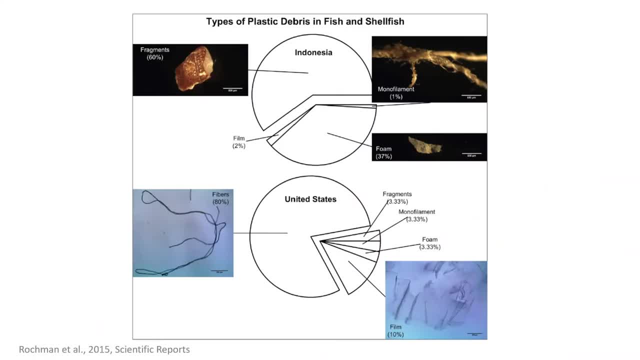 28 percent of individual fish and in 55 percent of all seafood species, so 55 percent of all seafood species. we find micro uh debris from the human activities. Similarly, in the USA anthropogenic debris has been found in 25 percent of individual fish and 67 of other seafood species, so 35 in fish species and 77. 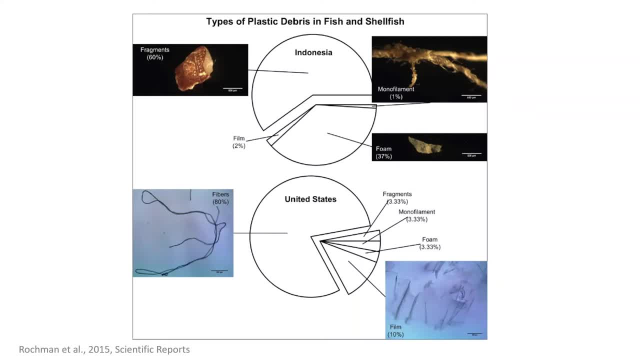 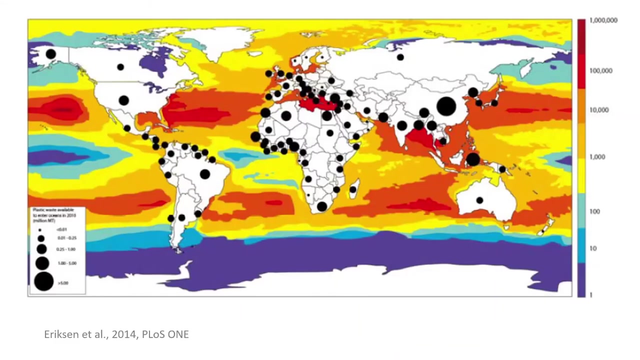 uh 67 in other seafood species. all of these anthropogenic debris recovered from fish in india is plastic, whereas in the USA this is mainly debris of fibers. therefore, variation in diverse types likely reflect different sources and waste management strategies between different countries and continents. i would say regarding the ocean, for sedimentation rates are low and 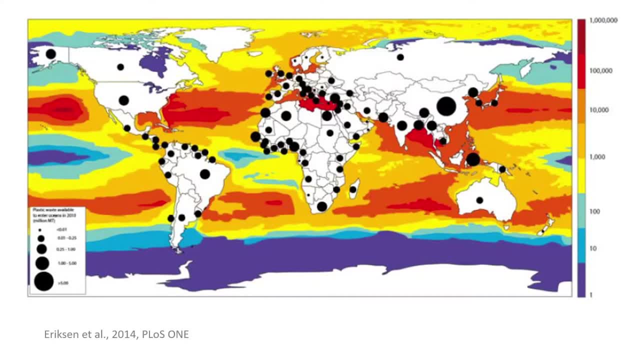 the anthropocene will be represented by millimeters in stratigraphic thickness, so this means that when plastic accumulates after a longer time period, new sediment will cover this plastic, and so forth and so forth, while the pressure will be high enough to compact this layer in into only a tiny millimeter. so, and uh yeah, and most of the c4 is bioturbated. 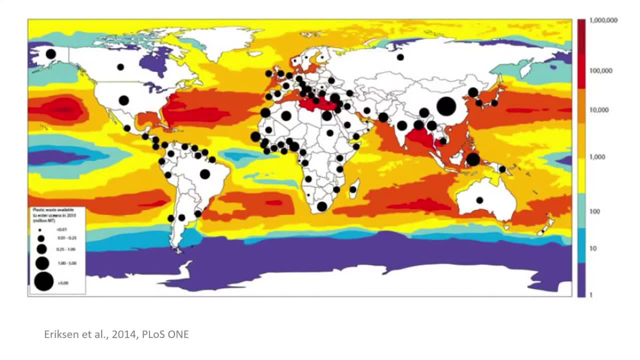 or mixed by benthic organisms. therefore the plastics or depth of a few centimeters will, like the rest of the sediment, it will be mixed with older deposits and separated from from them by a diffuse gradational boundary, so they will not be as a distinct marker, but 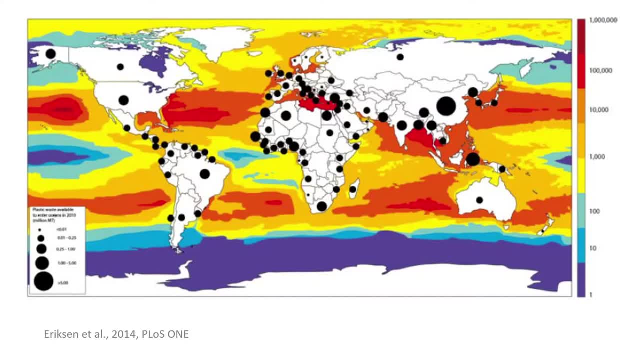 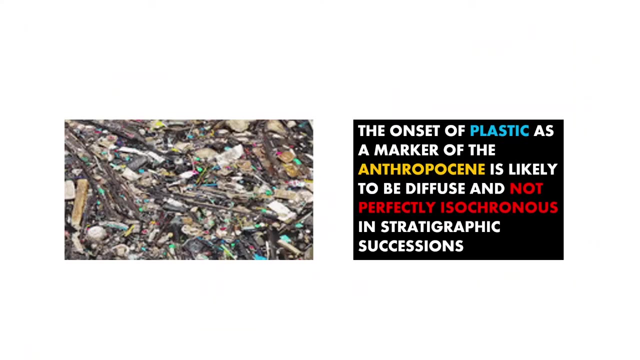 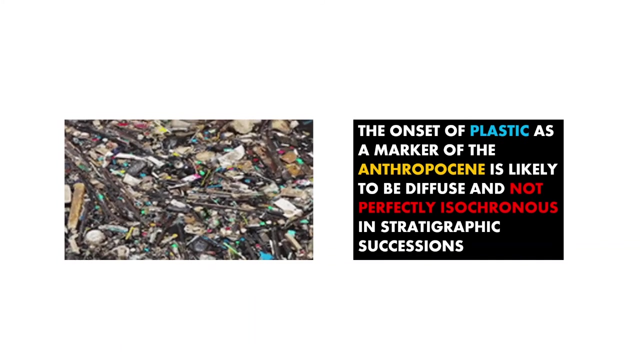 most likely a mixture with a other sediment, and this is one of the practical issues of applying a plastic marker or very short time period for the geological new epoch recognition, recognizing the exponential growth of plastics production since the 1950s. the onset of this marker of the 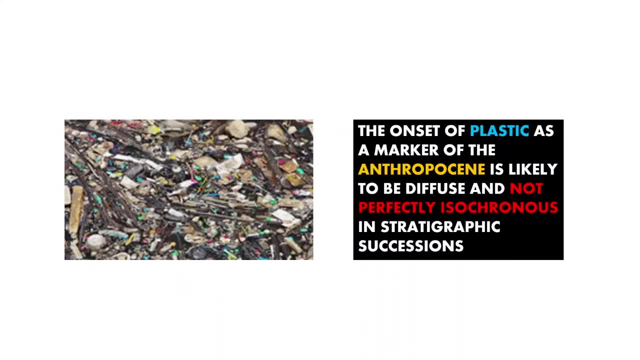 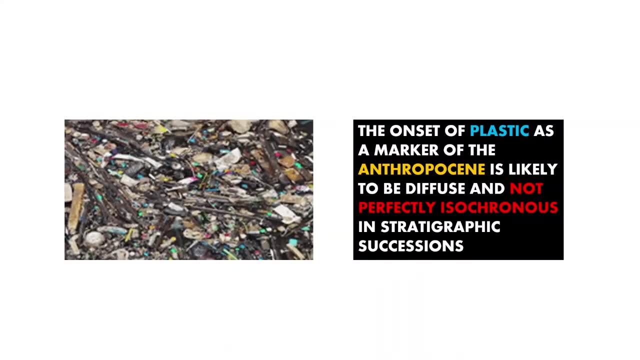 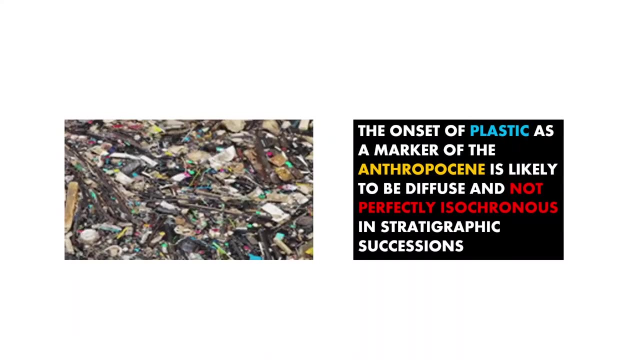 anthropocene is likely to be diffused and not perfectly isochronous and in a stratigraphic succession, so it will probably not be the best option what to choose. for instance, a significant presence of plastics in the marine and terrestrial environments was not recorded until the late 1960s to early 1970s. 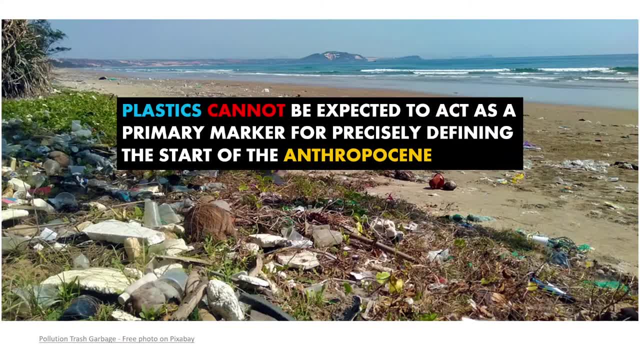 Therefore, despite their utility for plastical stratigraphy, namely recognition and characterization of the Anthropocene deposits, plastics cannot be expected to act as a primary marker for precisely defining the start of the Anthropocene. And that means that your concentration, distribution localities are not synchronous or homogeneous all over the world. 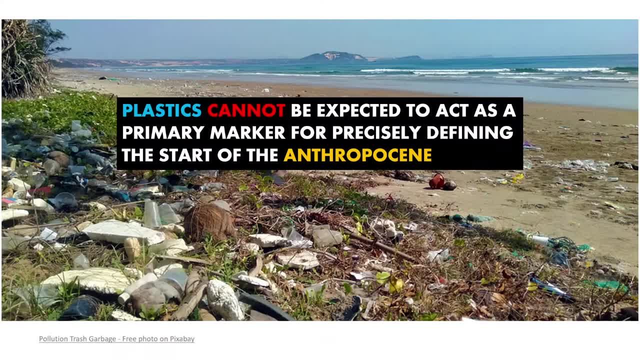 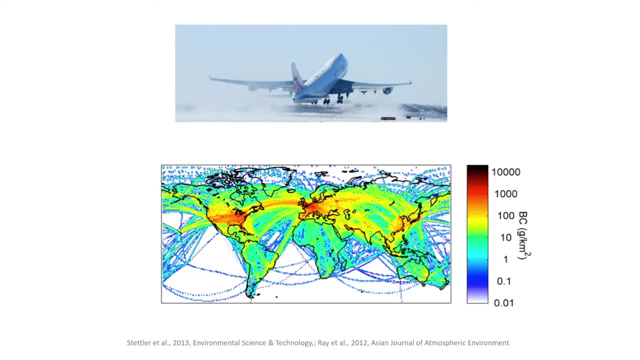 Because we have some hot spots where we can find plastic more and somewhere less, So that can be a challenge to use this marker as well. Air pollution, So aviation emissions, are increasingly significant contributor to anthropogenic climate change and global aviation emits about 1.04 billion tons of carbon dioxide every year And this represents 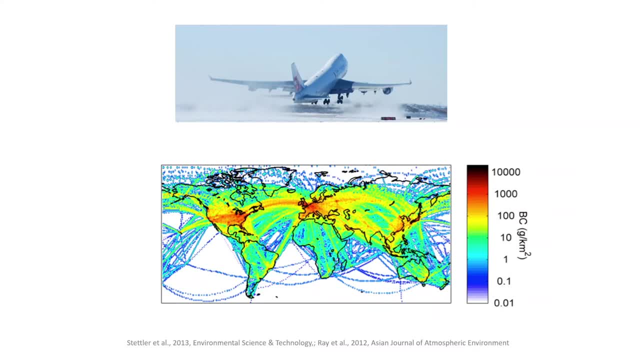 about 2.5% of total CO2 emissions per year, When to consider the full flight, which includes emissions from takeoff, cruise and landing. aircraft emissions impact air quality and emit small particles, which are basically nanoparticles. These particles, alongside chemical metals, 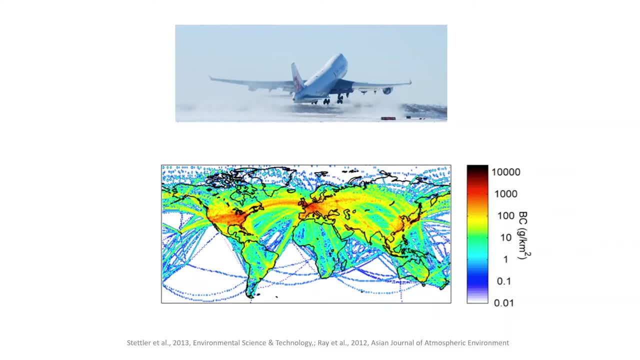 settle out on land and also in oceans. of course, There have been studies which indicate that these particles are more likely to be used as the key components of the Anthropocene compared to the other two. We can see that these particles are more likely to be used as the key components of the 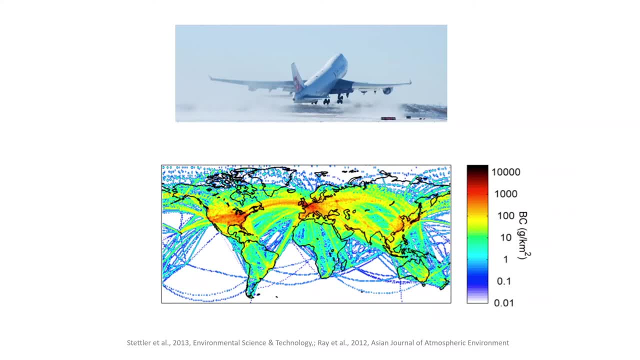 Anthropocene, And they are more likely to be used as the anti-pagetic markers, But it is not clear whether they truly would last long enough for coupling as a decent marker, And not to mention that their recognition within the sediment might be an issue Because their distribution, as you see, 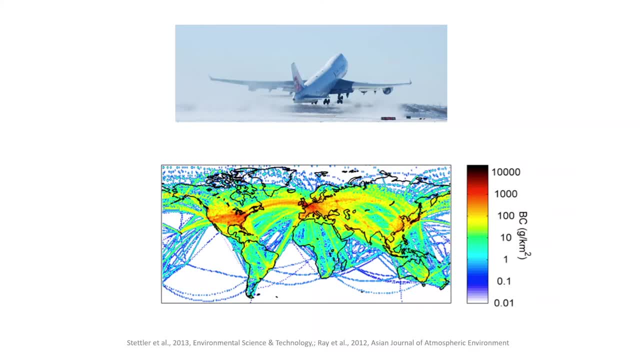 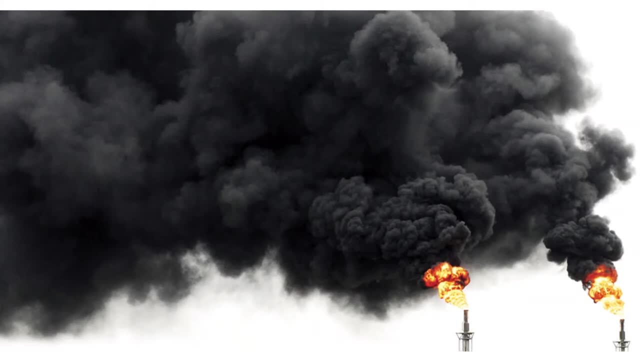 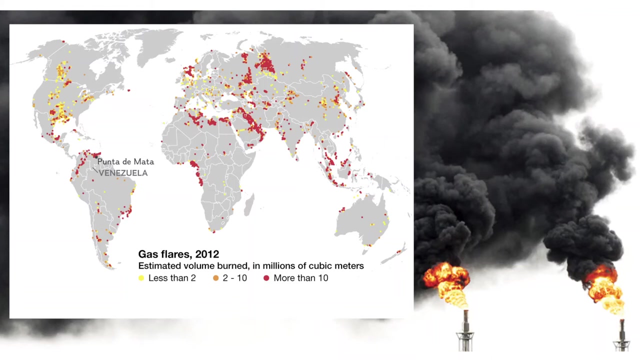 all locations. Well, air pollution is crucial and we see that in a few generations mankind is exhausting the fossil fuels that were generated over several hundred million years and the main oil and natural gas regions overlap and, as you probably know, then during the oil extraction process, vast 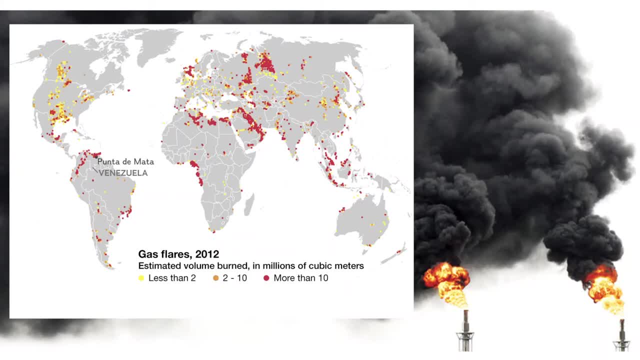 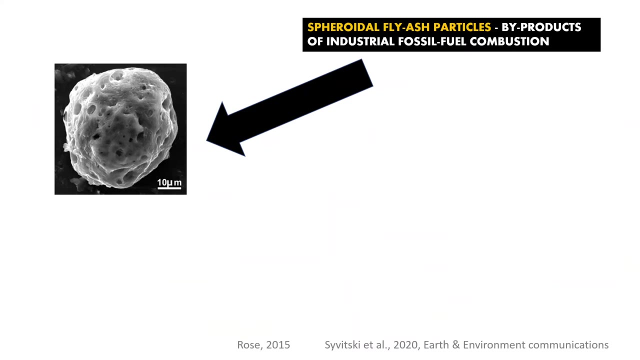 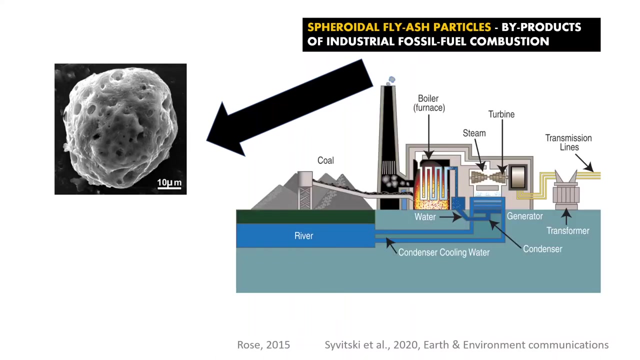 amount of natural gas coming out as a side product is burned, and these numbers, of course, are just staggering. Well, during the high temperature fossil fuel combustion, fly ash particles are produced and emitted to the atmosphere along with flue gases. These are two main particle types in organic ash. 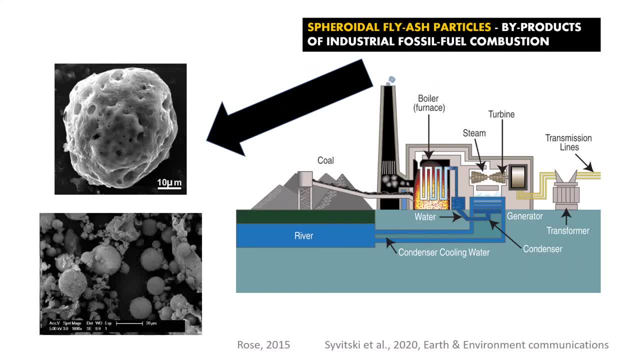 spheres which are derived from non combustible minerals present within the fuel and spheroidal carbonaceous particles, or SAP, which result from the incomplete combustion of the pulverized coal particles or oil droplets themselves and are a component of the black carbon. So we are 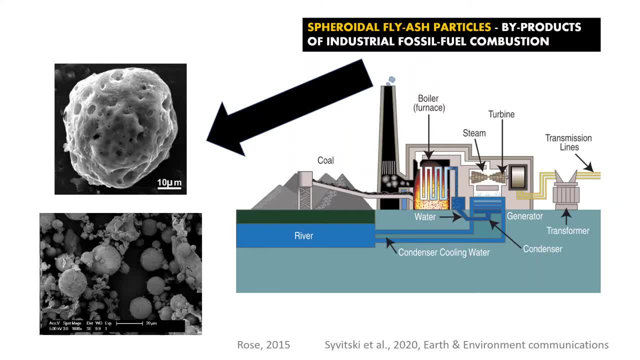 talking here about the black carbon pollution, which is basically air pollution. but they tend to also settle down somewhere and these particles again form during high temperatures, not like diffusing from the, from the cars or airplane. So we are talking about heating power plants. Well, they have no natural sources. due to this, 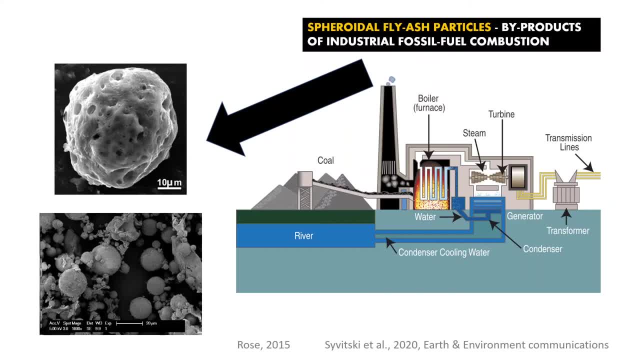 high temperature and their characteristic shape, color and morphology make them as excellent indicators of contamination from this environment. Let us not just look at our model here. There is only a few pictures, but here we have different写 source. Further, they preserve in a range of accumulating media, including 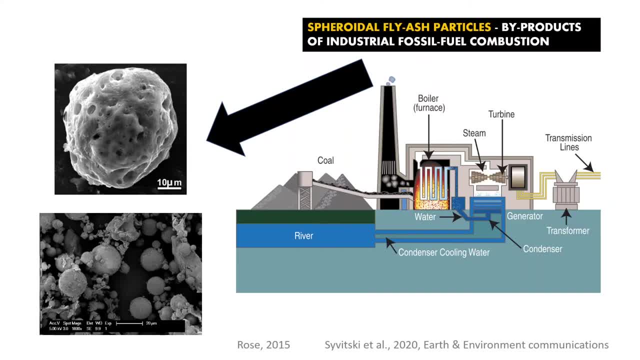 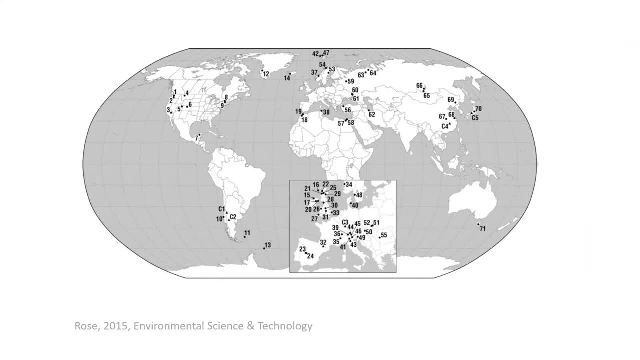 freshwater and marine sediments, peat and ice, So we can find them everywhere. The SCP data from 71 lakes across the world have been compiled in 2015, publication by Rose, and this study covers Europe, North and South Americas, Asia and one site South to Australia. The point is that across all these sites, 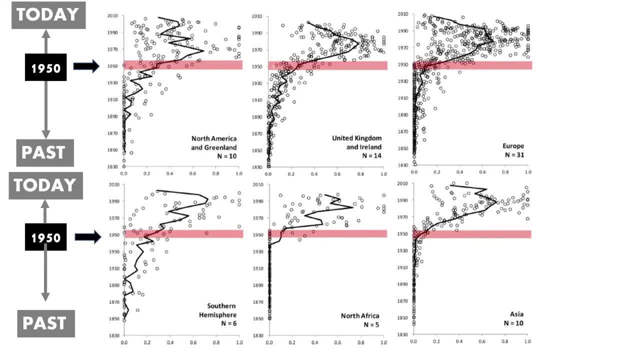 SCP record begins in the mid 19th century, with the rapid increase starting from 1950s, and this dramatic increase in SCP deposition is concomitant with many other indicators of great acceleration, as we call it, including the increasing, of course, primary energy uses, and is linked with the post-World War II. 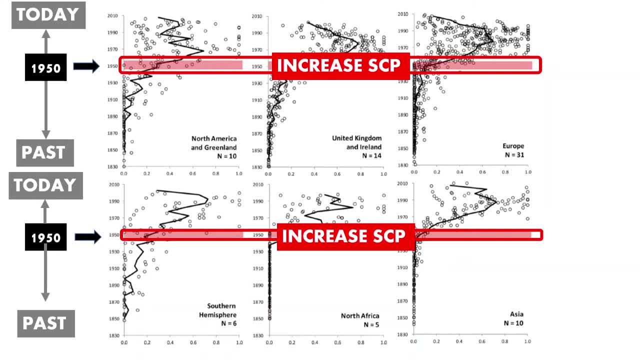 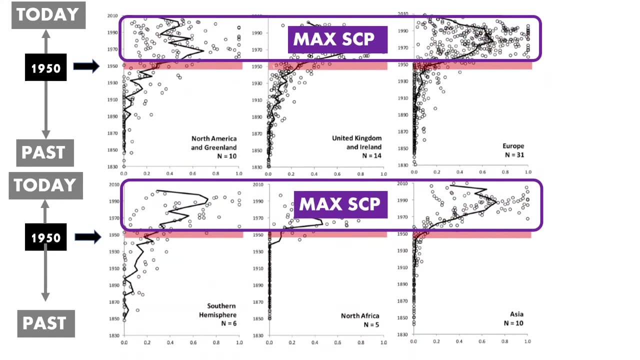 increase in the demand for electricity and the introduction of cheap fuel oil. The duration of this rapid increase varies between the regions because the SCP concentration peaks are often followed by decline in inputs. But the rise in SCP is about around 1950 and this is 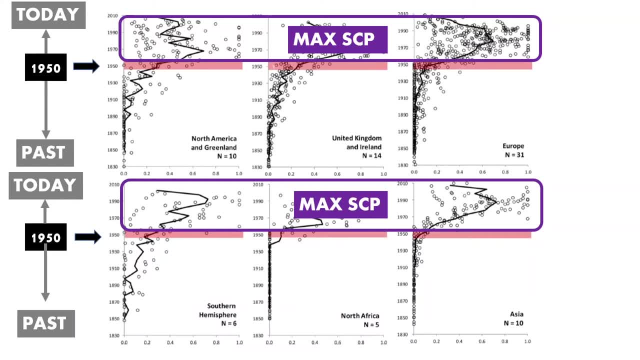 recognizable in all over the world. Yeah, there are several reasons for for decline in some regions after the peak is reached and, for instance, some kind of filter systems are a new technologies are used to applied also. the source of fuel has changed and the regional decline of heavy industry as well. therefore, 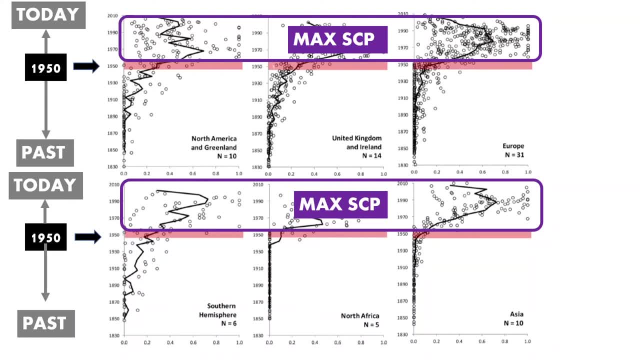 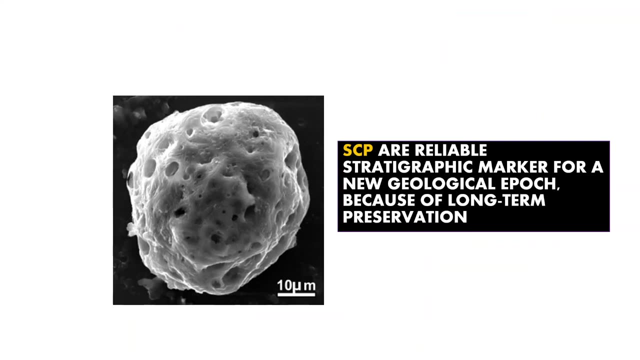 Therefore, while some features of SCP profiles vary regionally, the rapid increase in the 1950s appears to be a global signal which can be attributed to human activities. SCPs are a reliable stratigraphic marker for a new geological epoch. because of long-term 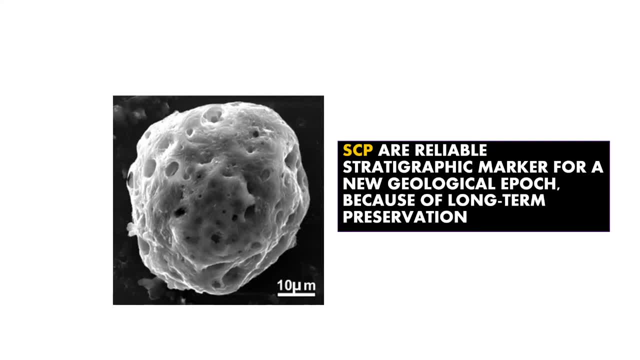 preservation. However, carbon-rich particles with bubble-like textures, thought to have been formed by bolide, impact into organic-rich geology around 65 million years ago before present, and have been observed at the Cretaceous-Paleogene boundary. These are thought to have been produced by low temperatures like 300 to 800 degrees. 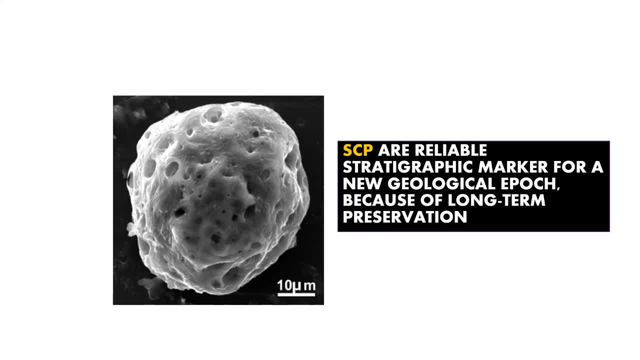 and they are still preserved. but, as I said, they are not exactly look-alike as SCP, but a similar type of particles. Therefore, the source of these particles might be promising in the terms that we can predict. Thank you If SCPs were to be preserved similarly well, and there is no reason to suggest that they. 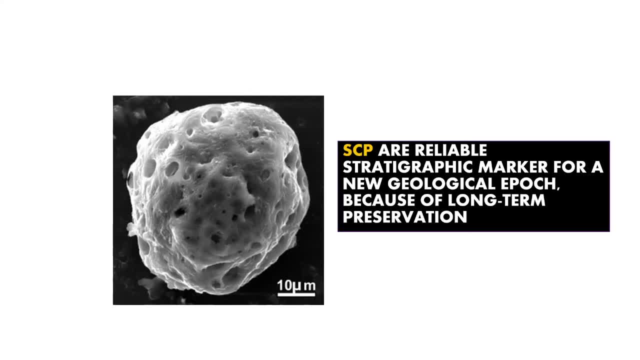 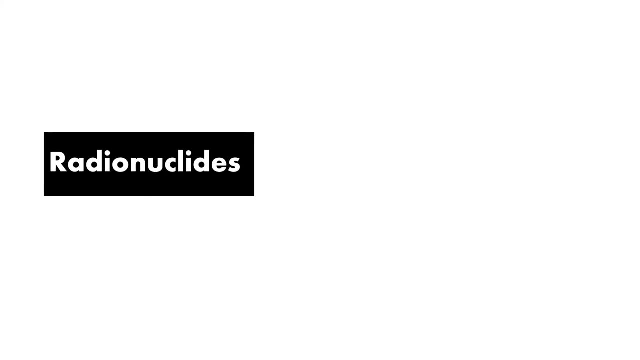 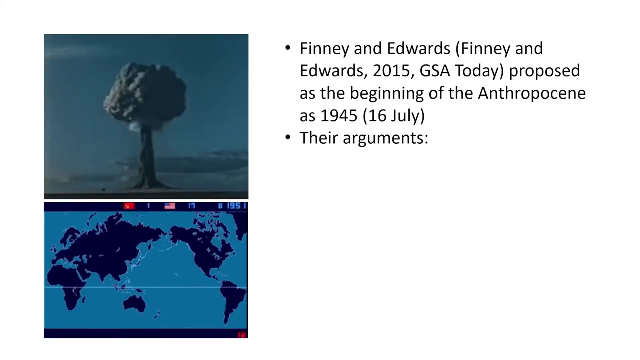 will not, then they would easily meet the criteria for a long-term stratigraphic marker. Next, one huge discussion field is about radionuclides. Finney and Edwards proposed as the beginning of the Anthropocene precise date: 16 July 1945.. 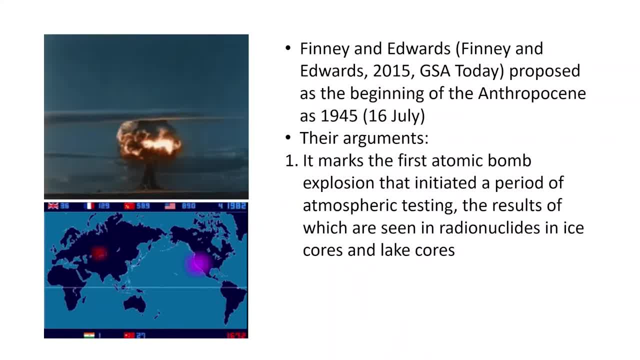 Their argument was that it marks the first atomic bomb explosion that initiated a period of atmospheric testing. The result of the atomic bomb explosion was the first atomic bomb explosion that initiated a period of atmospheric testing. This is not yet the case, but if you take the Demolition of the Disruptive sistemas in 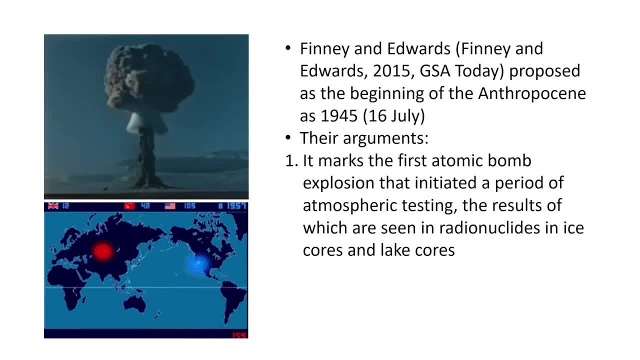 the end of the 14th century BC, after the beginning of the third-century BC, since the 15th century BC, manytwo or 15th century BC that we could see in radionuclides, in ice cores and lake cores. at least one human generation has passed, which is important for establishing. 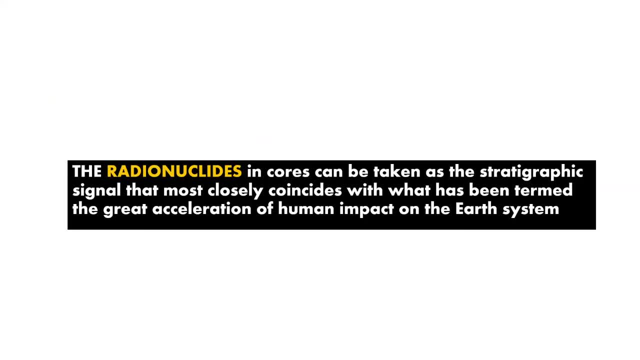 a stratotype. The radionuclides in cores can be taken as the stratigraphic signal that most closely coincides with what has been termed the great acceleration of human impact on the earth's systems. So again, great acceleration, So this term is widely used. 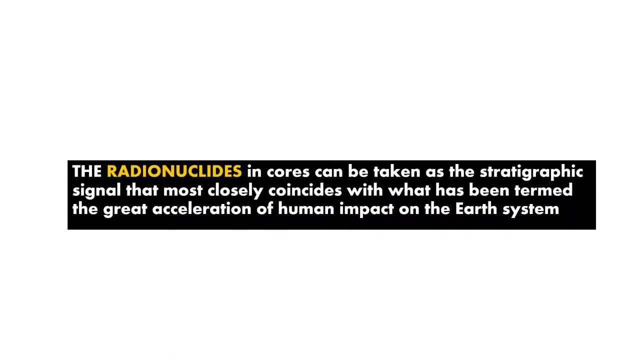 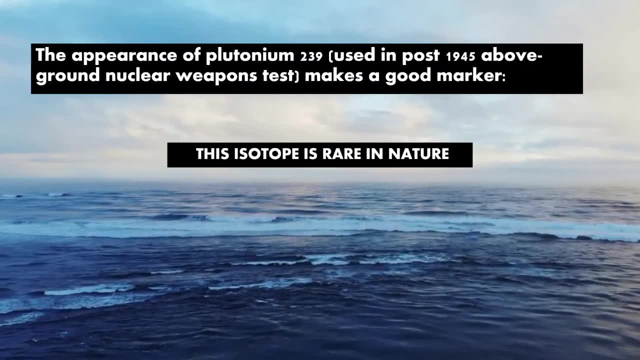 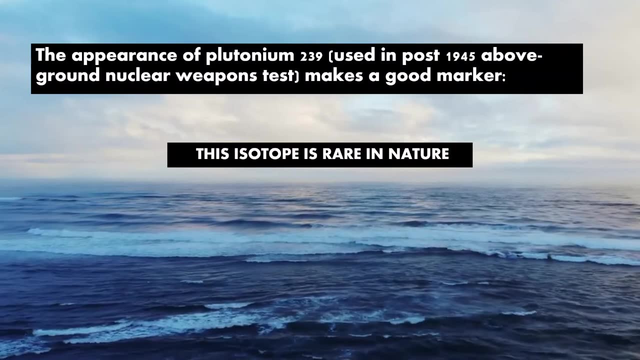 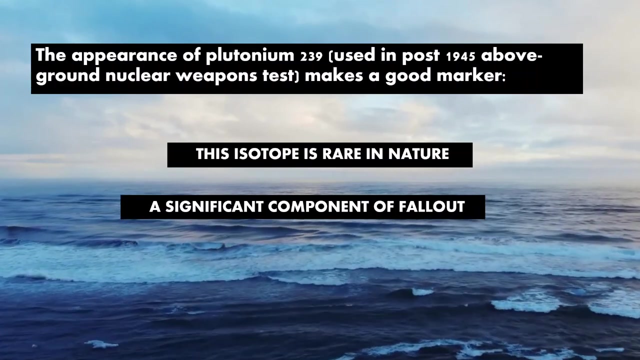 So next question, widely used when we consider human impact, Standard stratigraphic practice requires a significant, globally widespread and abrupt signature, and the fallout from nuclear weapons testing appears most suitable for this. The appearance of plutonium-239 makes a good marker. this isotope is rare in nature. a significant component of fallout, a stable marker in layers. 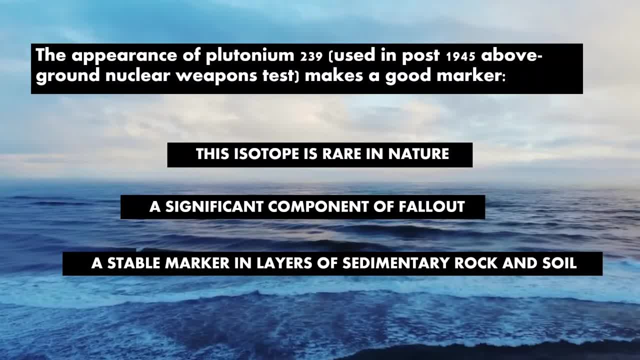 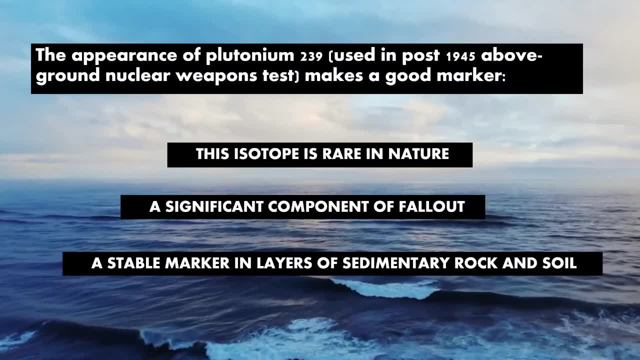 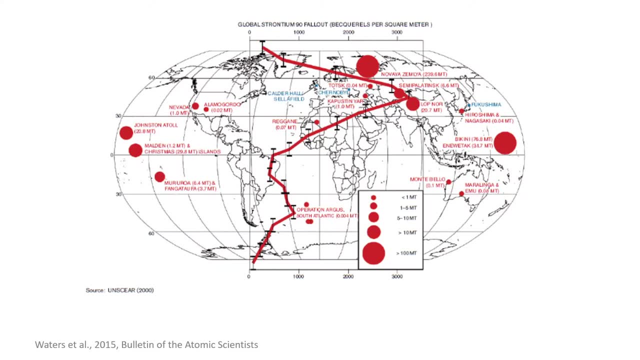 of sedimentary rock and soil On a global scale. the first appearance of plutonium-239 in sedimentary sequences corresponds to the early 1950s. It can be used to define the Anthropocene sites located between 30 and 60 degrees north of the equator, because there 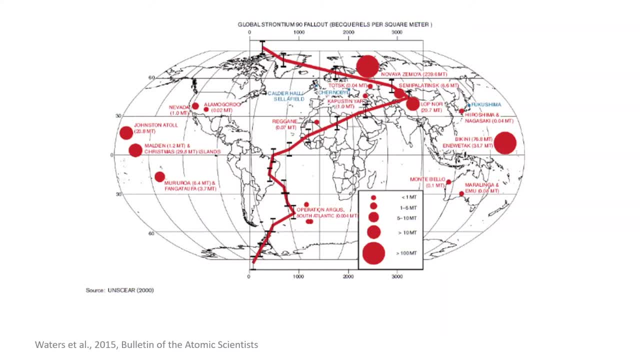 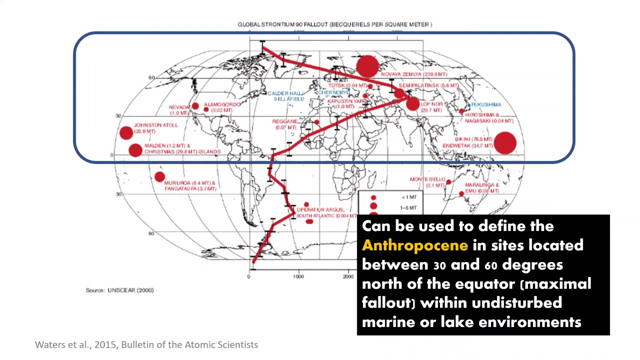 it was maximum fallout for these testing episodes and probably only within undisturbed marine or lake environments these radionuclides can be detected. But again, if we consider the worldwide evenly distributed signal, then you see there are some mismatches between the both hemispheres And the long half-life of plutonium-239,. 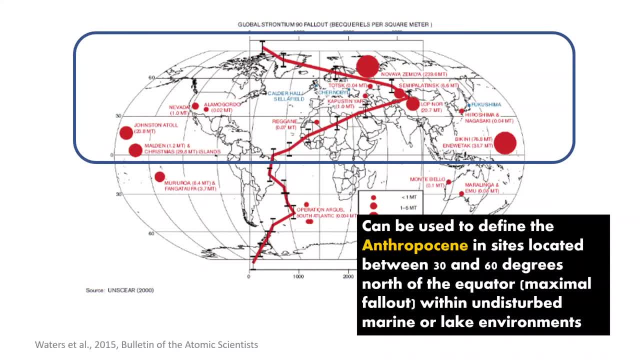 which is 24,000 years, makes it the most significant of the two. The long half-life of plutonium-239,, which is 24,000 years, makes it the most persistent artificial radionuclide detectable by modern mass spectrographic. 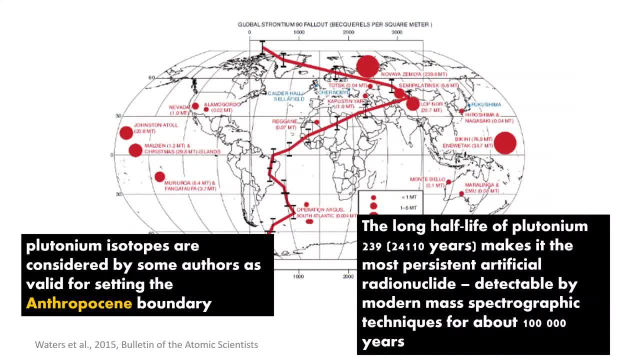 techniques for about 100,000 years. Whether it's enough, well, that's a question. 100 years in geological terms is clearly nothing but well. there are discussions that we can use this one at least to support Anthropocene boundary. Plutonium-240, also a. 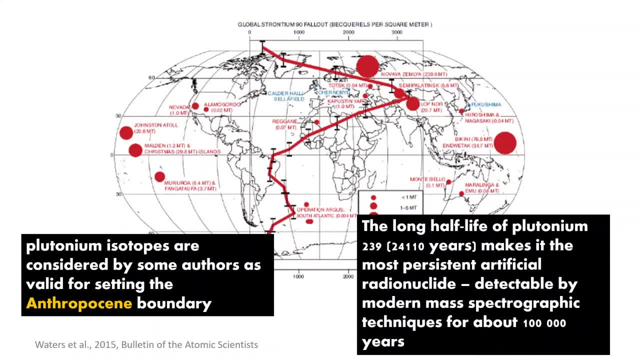 product of nuclear weapon testing is less abundant and has a shorter half-life, hence not so good for a marker. Therefore plutonium isotopes are considered by some authors as valid for setting the Anthropocene boundary. But the question, of course, when we consider 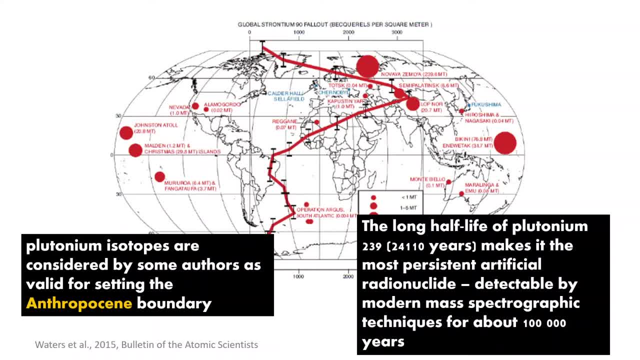 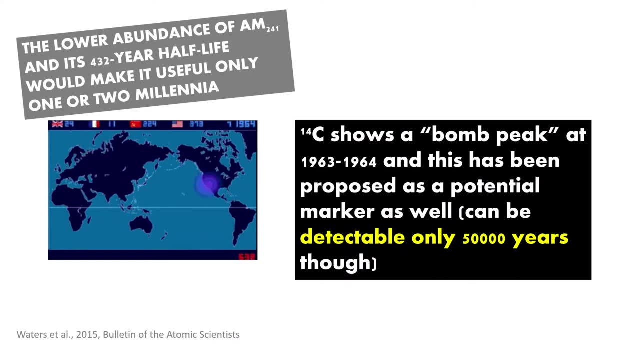 this half-life of these elements and radionuclides, then there is some shortage. The short half-lives of caesium and strontium limit their potential to serve as geologically permanent markers, which are again different kinds of radionuclides. 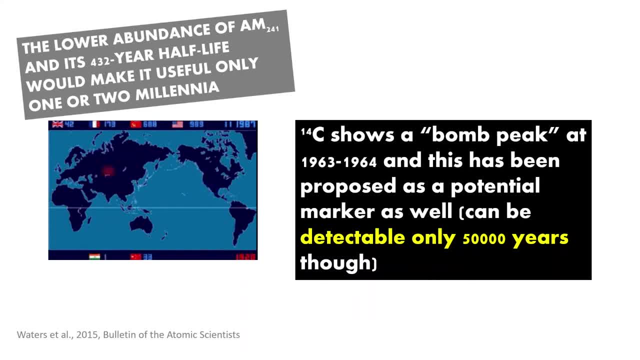 Then amritium-241 has a deeper water distribution than plutonium, being more readily transported to the bottom of deep oceans on signing organic particles, and so may be a more suitable signature in the undisturbed deep-water environments. However, the lower abundance of amritium and its only 432-year half-life would make it useful only for 1,000 or 2,000 years. 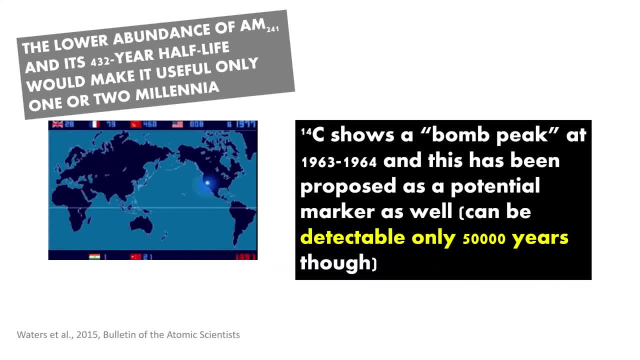 C-14 shows a bump peak at 1963-1964, and this has been proposed as the second peak. There's a potential marker as well and can be detectable only 50,000 years ago. So radionuclides are promising, but their half-lives and longevity and detection from the sediments is the major concern. 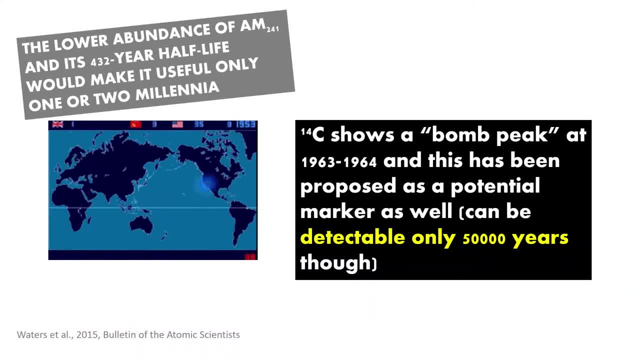 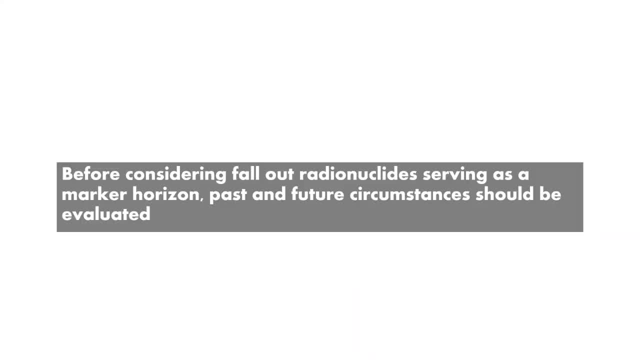 How can we detect and why we should use them if they are not traceable after, let's say, 100,000 years, Which, from the geological point of view, is then questionable? Before considering fallout radionuclides serving as a marker horizon, past and future circumstances should be evaluated as well. 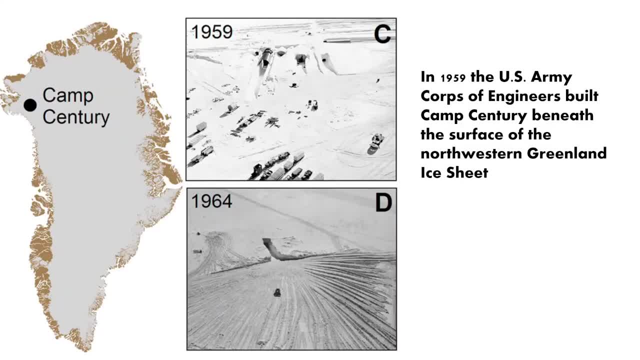 For instance. one example: The advent of long-range aircraft capable of deploying nuclear bombs drew military attention to the Arctic, which was the shortest route between the Arctic and the Pacific. which was the shortest route between the Arctic and the Pacific. It is known as the shortest route between the US and USSR. 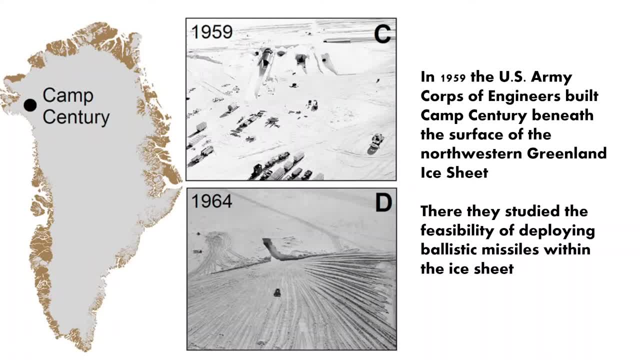 During the Cold War. in April 1951, the US and Denmark signed the Defense of Greenland Agreement of building three airbases in northwestern Greenland. In 1959, after several years of intensive ice sheet research, the US Army Corps of Engineers built a camp-centry which was excavated at 8-m depth. 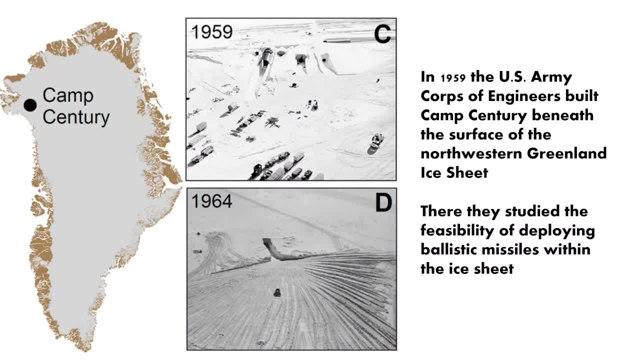 ice sheets, porous near surface fern, so a specific fern it's a. it's not like a ice sheet yet, but it's in in the middle. so therefore it's porous near surface fern, not ice. what we considered true ice. it's going there, but not yet. and well, these engineers there, they studied the 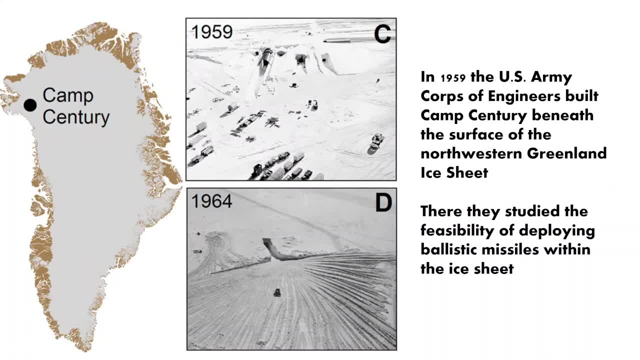 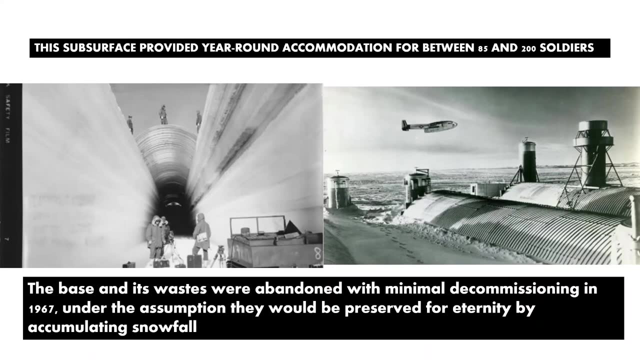 feasibility of deploying ballistic missiles within the ice sheet. so for the military purposes, this subsurface provided year-round accommodation for between 85 to up to 200 soldiers and was powered by a portable nuclear generator and logistically supported by pulling supplies across an hour snail. 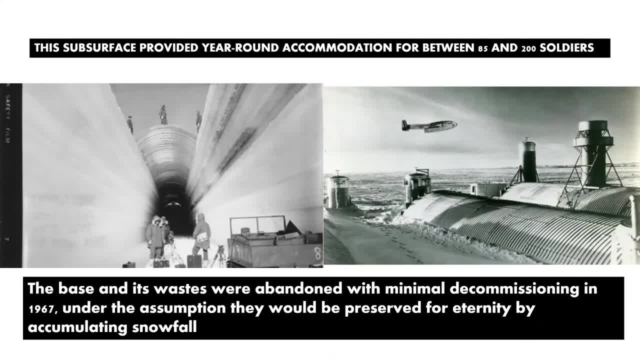 over snail trail and this project called ice warm and was it terminated in 1963 because it was rejected, too costly to not efficient enough, and year-round operations at camp century keysed or ended in 1964.. seasonal operations continued until 1967, but it was not year-round operations anymore. 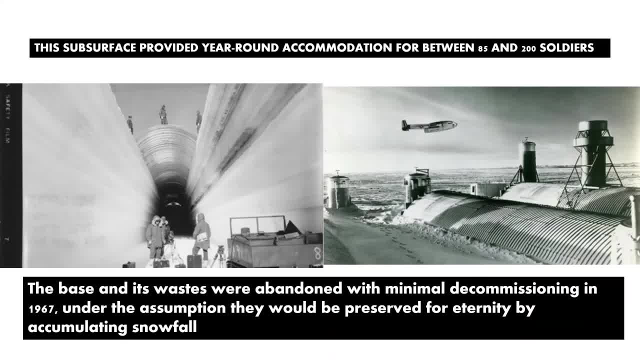 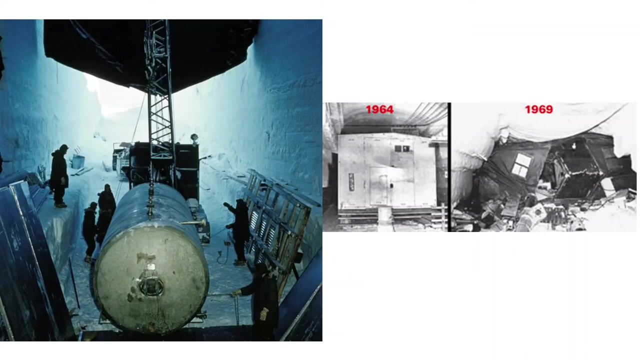 great بعد 1st. in the secret service they assumed the snow will cover this base and everything will be captured in a capsule. so everything will stay put there and nothing will change. The last reported visit to the abandoned camp sanctuary site was in 1969. Aside from the reaction chamber of the portable nuclear generator, 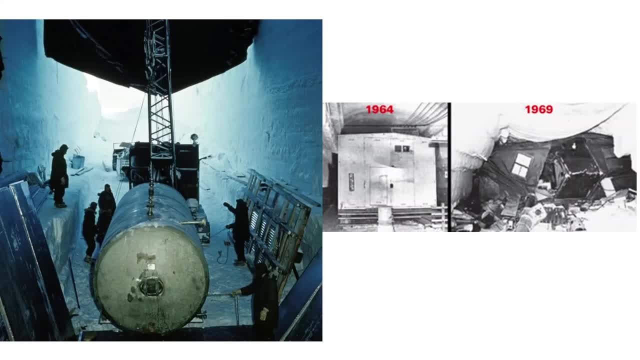 which was removed for destructing testing later. all infrastructure remained in the collapsing tunnel network after the 1969 survey. So the picture from 1964 and a few years later. obviously there are tremendous changes. everything is collapsing. So the camp sanctuary tunnel network. 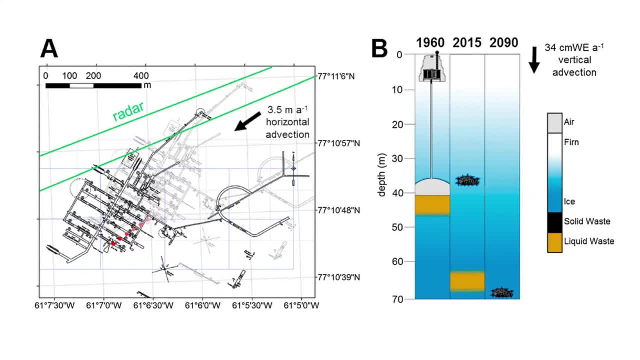 covers approximately 55 hectares and basically it is the only one in the world that can be seen in such a way. Based on modeled vertical advection rates, the majority of solid waste is now likely buried at approximately 36 meters depth. Due to the relatively efficient movement of liquids within permeable fern, the burial depth of 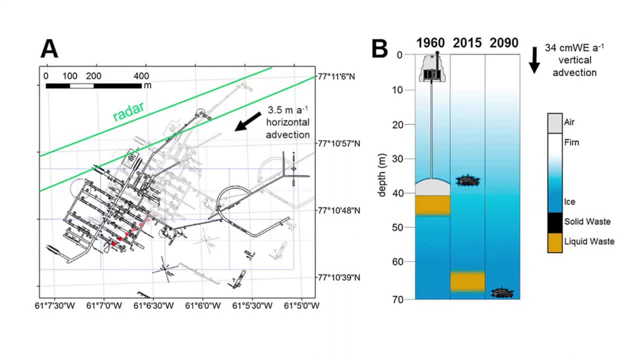 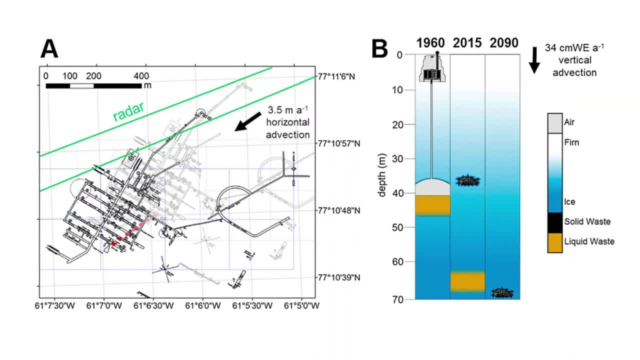 And may even remain liquid to date, although the tanks have likely ruptured. so that means indeed this kind of setting has now is covered by the ice, but it is not in that shape what it was when they left the site, and the fuel in these conditions are specifically. 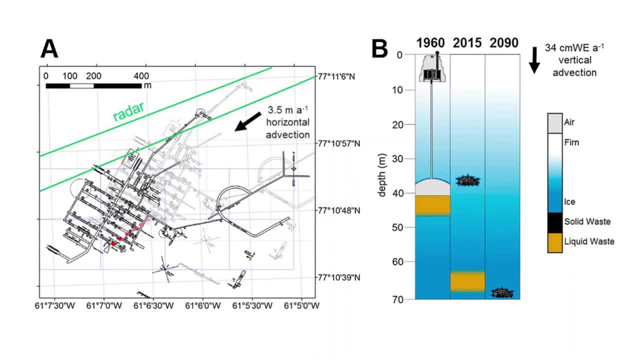 made to not freeze and therefore it's liquid still. but what has been assumed? that these tanks where the this fuel was kept? it's probably they have been broken and the fuel most likely has been now within the ice contact. An independent airborne ice penetrating radar observation system is now in use. 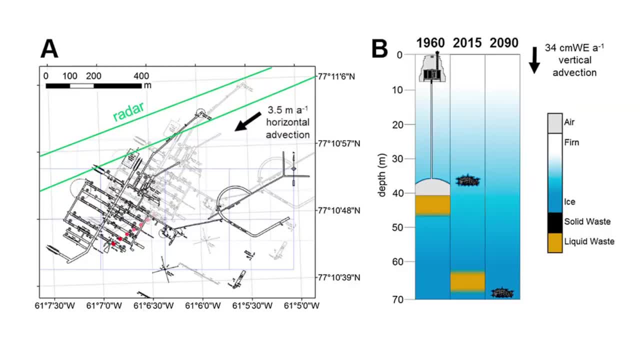 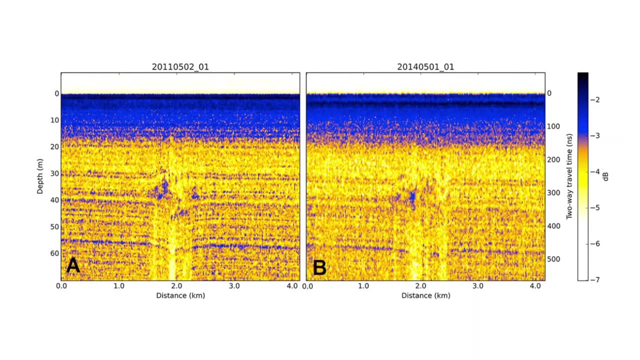 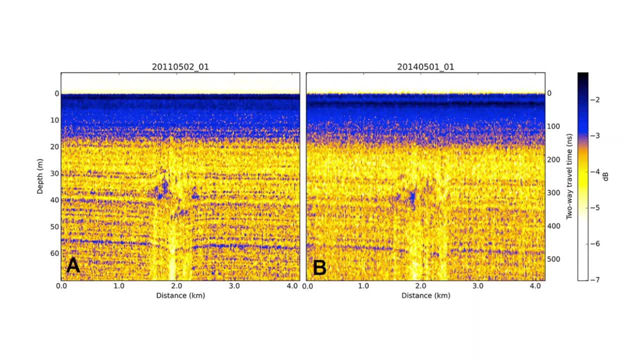 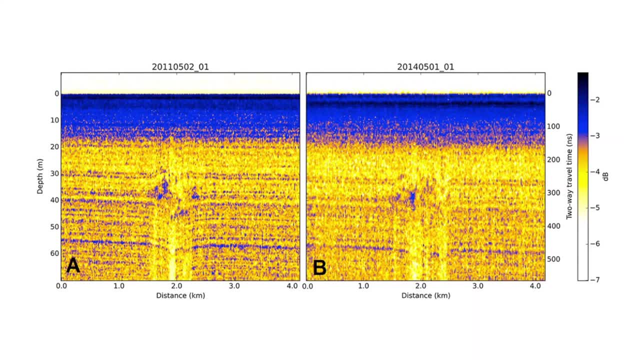 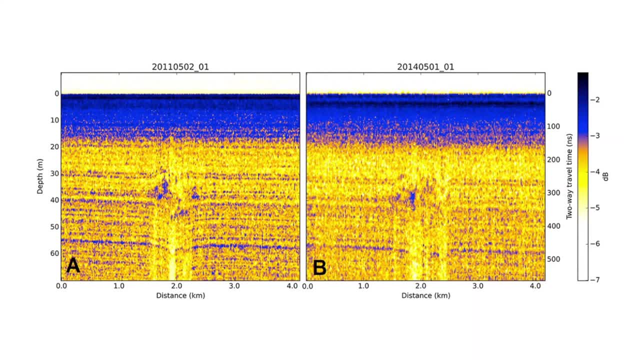 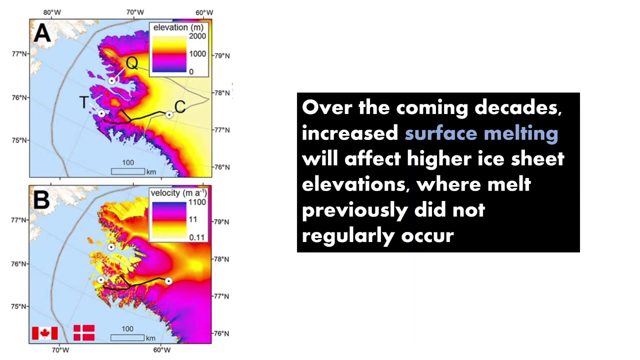 The radar observation system is now in use, So this means that we might see that this kind of object will get even deeper over the time. Since the 1960s, however, the scientific community has recognized the Greenland ice sheet to be more sensitive to climate forcing than previously thought. 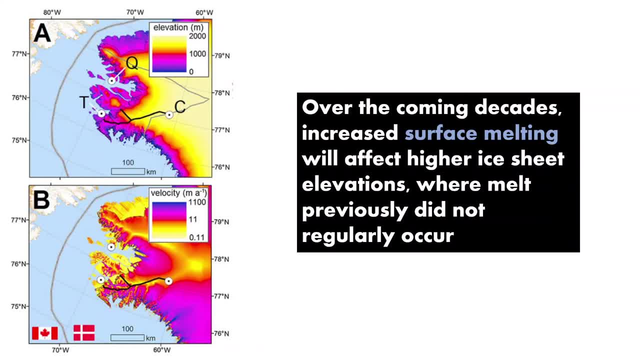 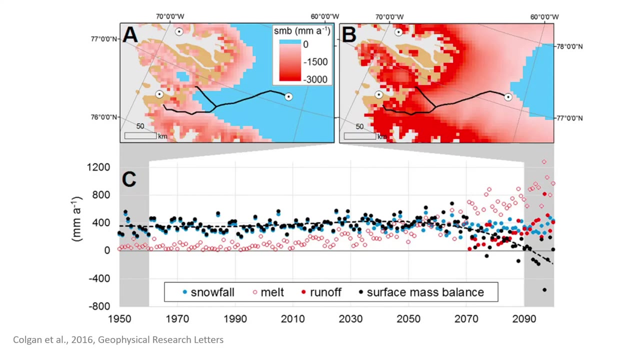 If to compare between 1900 and 1983 and the recent climate change, Greenland ice sheet has accelerated mass loss, So Greenland is having less and less ice and that might be some kind of issue also for this certain kind of example with these wastes of different origin. 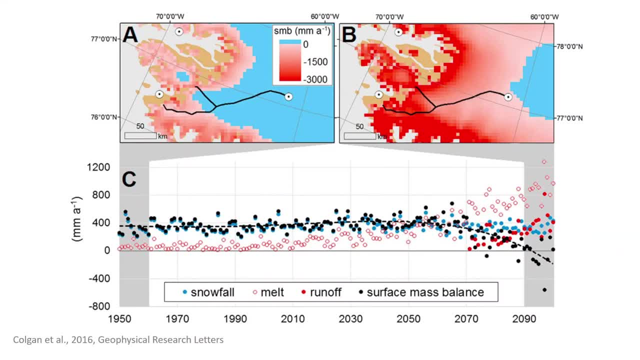 Given an antepassated to water Kind of solid waste depth in, let's say, 100 years from now, at 6744 meters, We can say that it might be the melting reason which then could expose waste at the ice sheet surface. 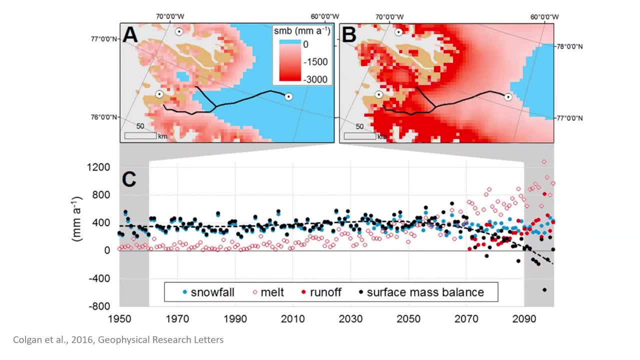 However, melt water can interact with the ice sheet With a deep fern more rapidly. We are vertical percolation, So observations indicate that surface melt water can percolate downward 10 meters through fern in a single summer melt season. So therefore it's a concern that it either either will be open after the ice will melt from the top or the melt water flow downwards. 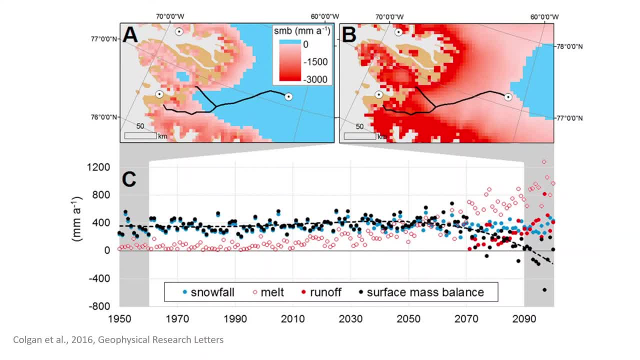 And so Downwards can increase the speed of movement of ice sheet itself And or Kind of Kind of run off of these chemical elements might easily go into the North Atlantic Ocean And abandoned US military base in the melting Greenland ice sheet may expose oceans to toxic pollutants by the end of the century. 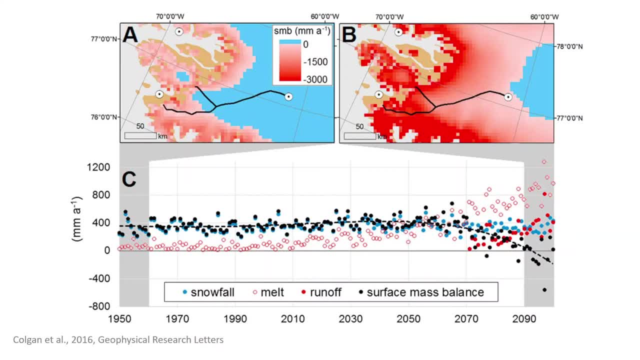 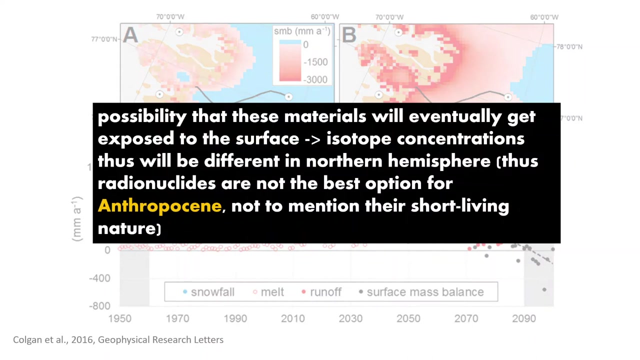 As I mentioned. Yeah, So ballistic missiles and other chemicals, radionuclides and toxic pollution is there, And this is only one example about which we now know. There might be also other examples- And many tons of toxic waste remain buried under the ice and continue to be an environmental concern. 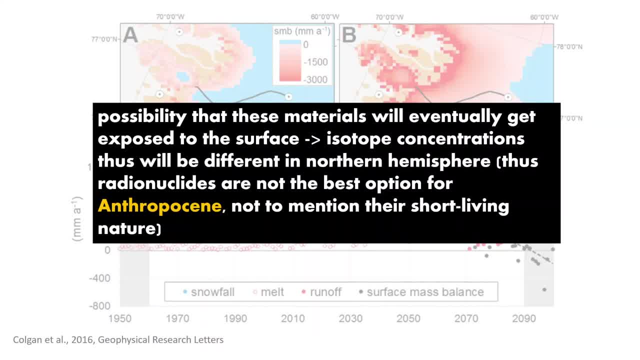 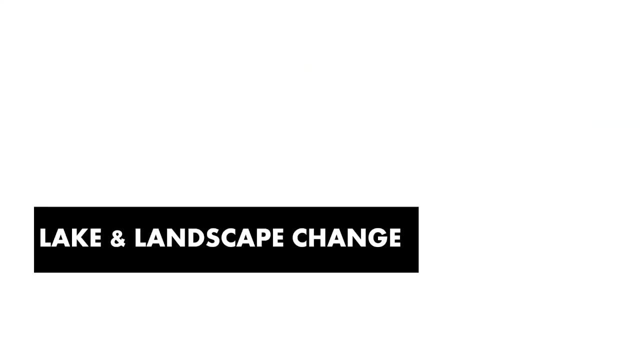 Particularly with The general trend of ice mass decreasing and the possibility that these materials will eventually get exposed, exposed to the surface, And therefore I still concentrations. Those will be different in Northern Hemisphere. Therefore these signals of human activities are not fixed in. 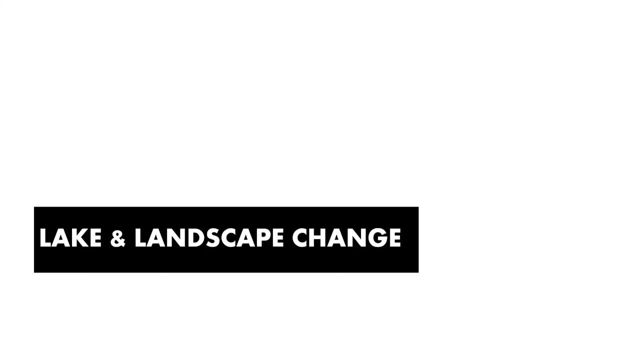 In one event, but might be Catastrophes Such as Fukushima, for instance, In Japan, Where we have Natural hazards all over the region. Therefore, the signal of radionuclides is probably Not the best idea to use for the Anthropocene had. defining the Anthropocene. 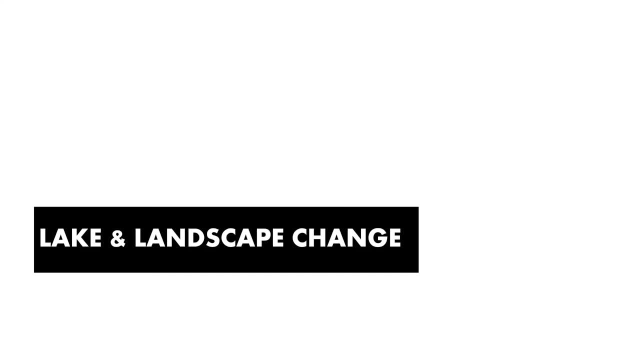 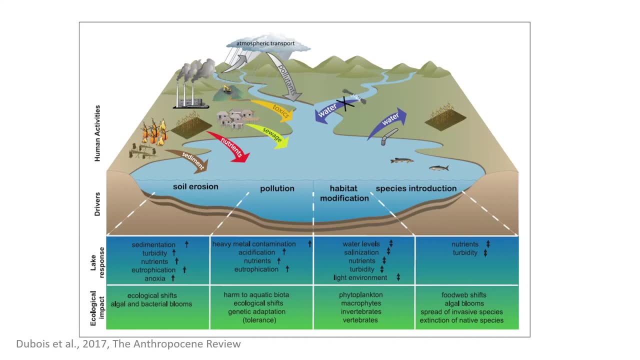 The next one is the lake and landscape change. Of course, a anthropogenic effects are also well illustrated By the history of biotic communities that will leave remains in lake sediments. The effects documented include modification of the geochemical cycle In large freshwater systems and occur in systems remote from primary sources. 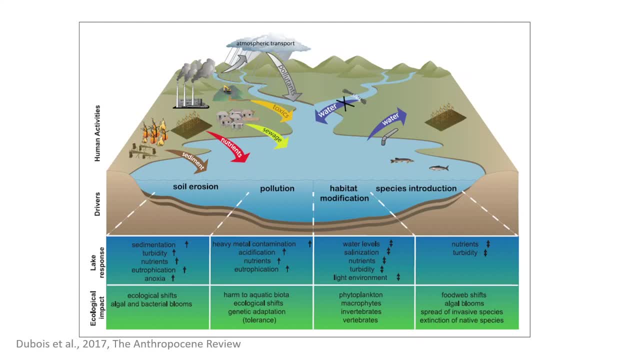 Surrounding catchment is tightly linked in this case- And I have been giving also some examples about the lake- responses to different kind of These can be Influences, How, for instance, algae community changes over the time Or under a different kind of pressure scenarios. 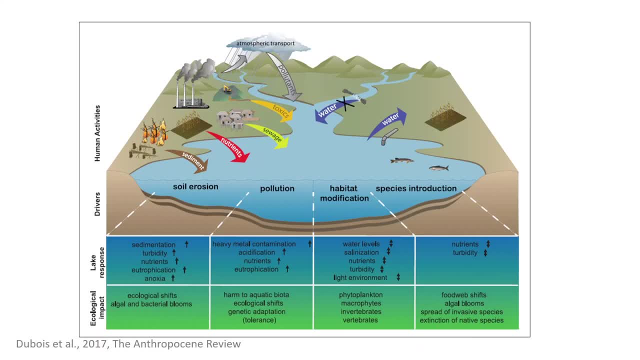 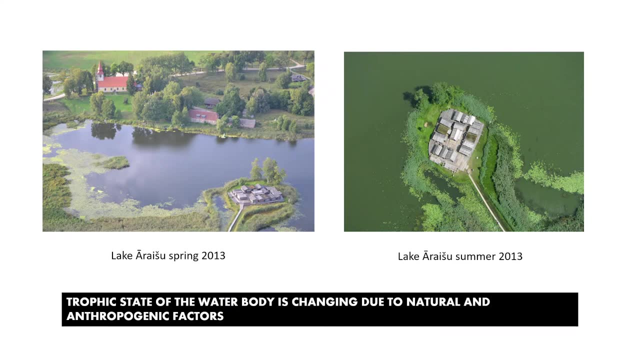 Trophic state of the water body is changing due to natural and Antropogenic factors, for instance Lake Arashi, Which is located in central Latvia, Central Northern Latvia, Then we can see that it still is polluted today In the 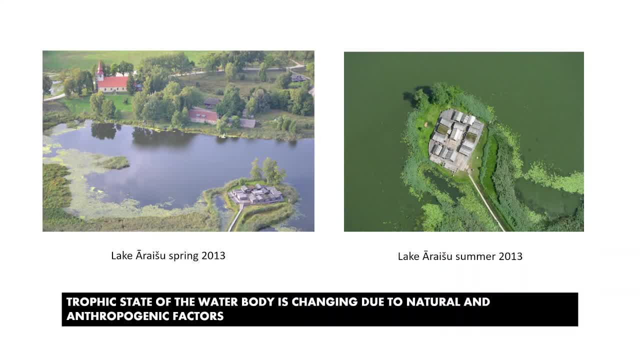 In the sense that humans have started to live there during the Iron Age And since that This Human pressure Related impact on the lake ecosystem has been Never released. So the lake still continues to Attract human impact Through various ways. 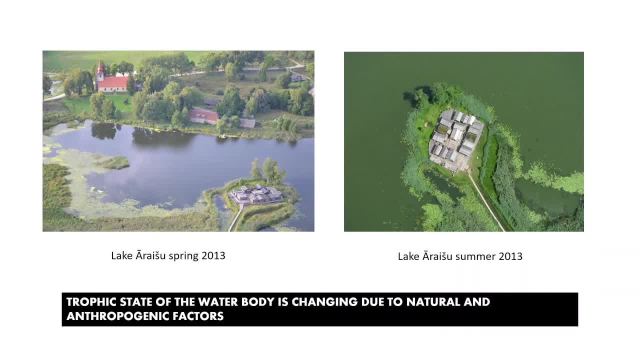 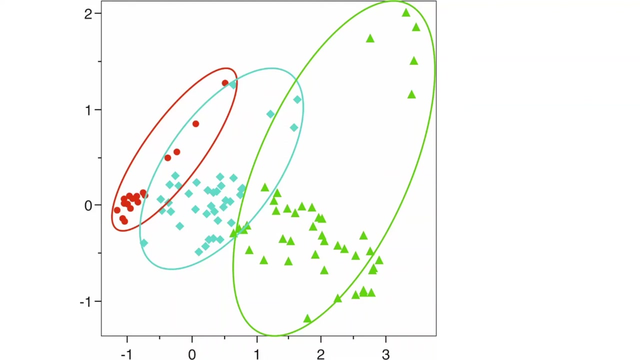 And this is an issue Worldwide- And Different Point of sources from A cattle breeding and Manuring of agricultural Activities around us, Around the lakes, can be traceable. And If to look closer to the territory of Latvia, then our analysis indicates significant shifts. 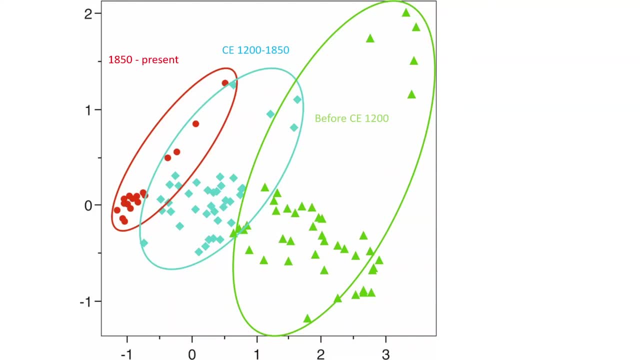 In algal composition in our lake since 1200 AD. Therefore, we argue that the reference conditions for this Lakes can be assigned with the age before this time. Therefore, all other changes affecting lake ecosystems are on top of that And it is not clear. 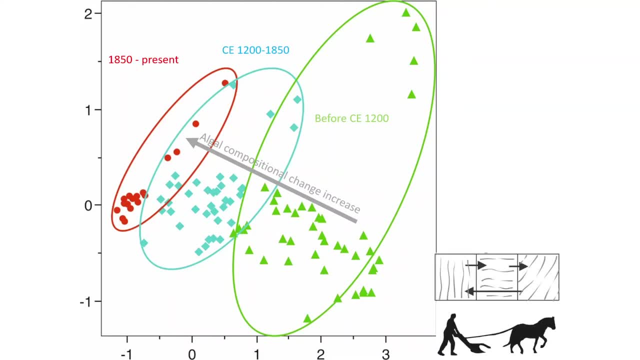 Why, then, 1950 would be the beginning of the Anthropocene? Because we see that the lakes and Water bodies and landscape has been modified significantly already before this time, 1950.. Any of these changes are recognizable From the sediments.